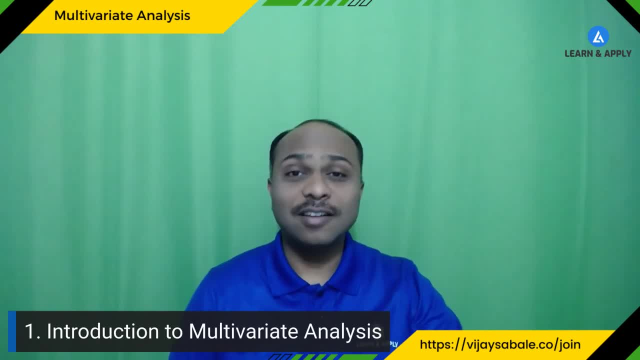 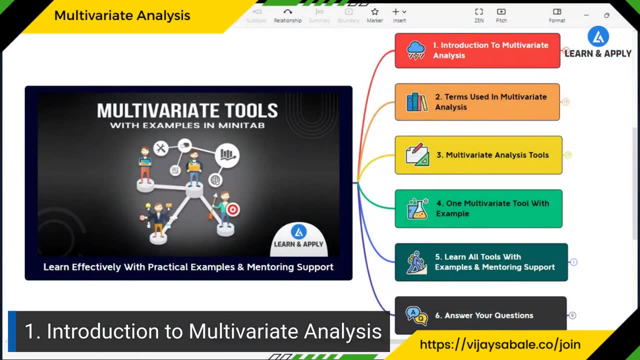 can put that into the chat box and I'm ready to help Answer all your questions. Okay, so the first topic is introduction of multivariate analysis. So let's go into the detail of it and let's understand what is this multivariate analysis first. okay, Now the today's learning is going in stage wise. that means we are going to understand. 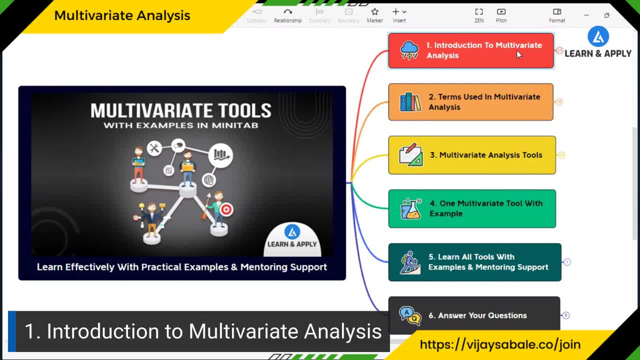 first, what is this multivariate analysis? then we will understand what are the various terms and concepts into the multivariate analysis and why it is important. because when we are going to learn the multivariate analysis, we are going to learn the multivariate analysis. to interpret the results, we must know all the concepts into the multivariate. Then, third in third, 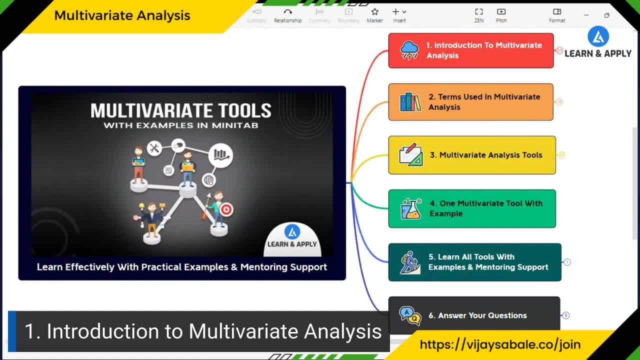 part, I am going to explain what are the various multivariate tools that are available and I'm also going to explain one of the multivariate tools with help of practical example. into the fourth part, Into the fifth part, I will explain what is the methodology by which you will learn. 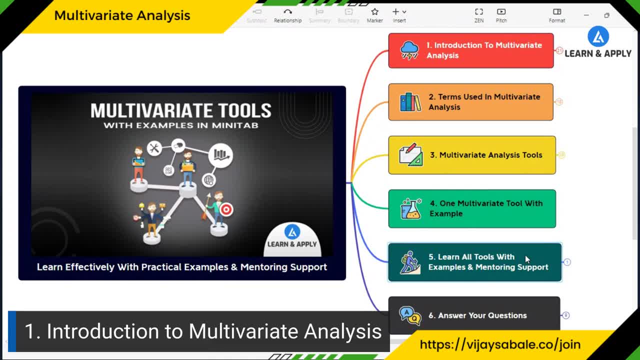 all the multivariate tools with help of practical examples and my mentoring support, and at the end of the third part, I will explain what are your questions and what are the answers to all that questions. okay, So let's dive into the first part, which is introduction to multivariate analysis. 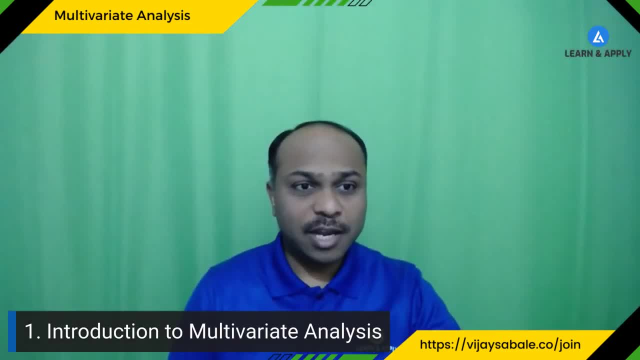 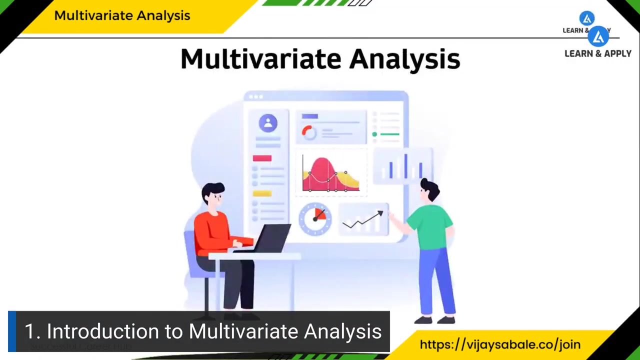 So let me show you the screen. meantime, if you have any questions, you can put that into the chat box. Let me share with the screen. can you see my screen? Yes, great, thank you. So the today's topic, as I already explained, is a multivariate analysis. You 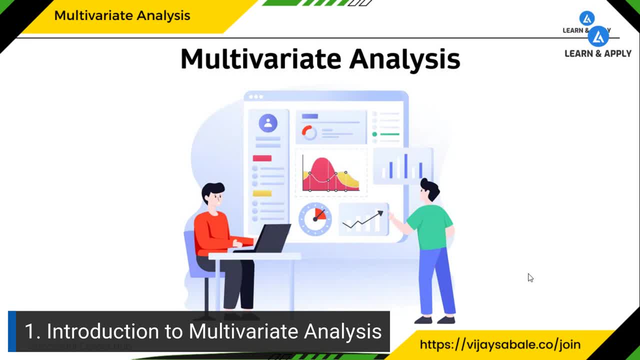 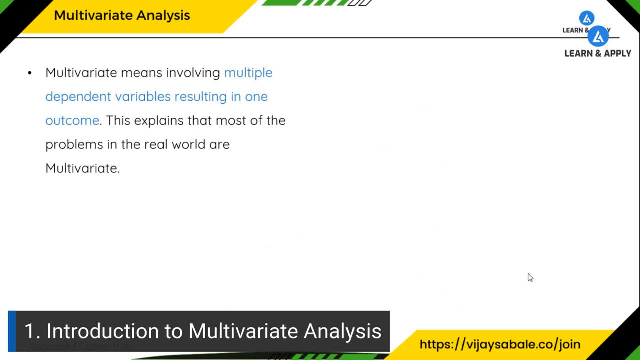 can see the picture, the multiple factors we are going to study at one time. Now let's go into the detail and just understand the basics of it. What is a multivariate? Multivariate means involving multiple dependent variables resulting in one outcome. That means one outcome or one result. 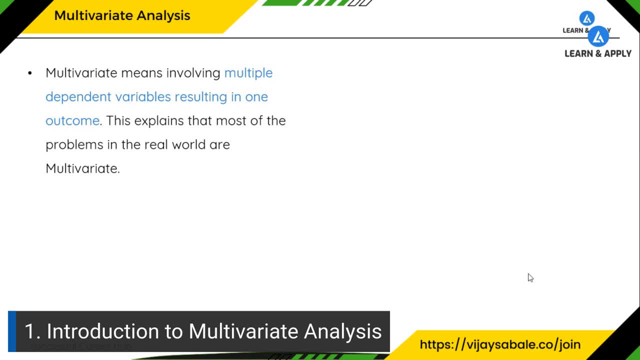 that we are going to see is the outcome of the multiple dependent variables, resulting in one outcome of many dependent variables. So we are going to understand what are these dependent variables? This explains the most of the problems in the real world are multivariate. For example, if we take the 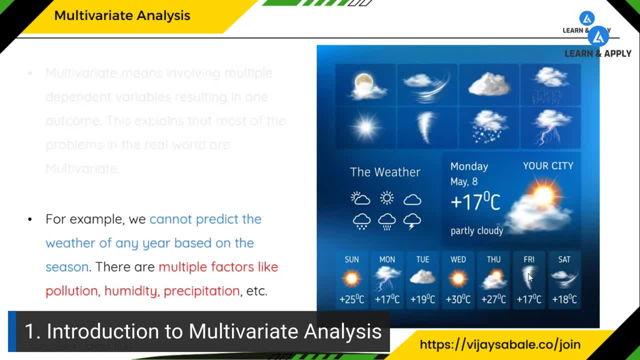 simplest example of weather. we cannot predict the weather of any year based on the just season right, because there are multiple factors like what is the pollution, what is the humidity, what is the precipitation, and there are many number of factors that needs to be considered to predict what we are. 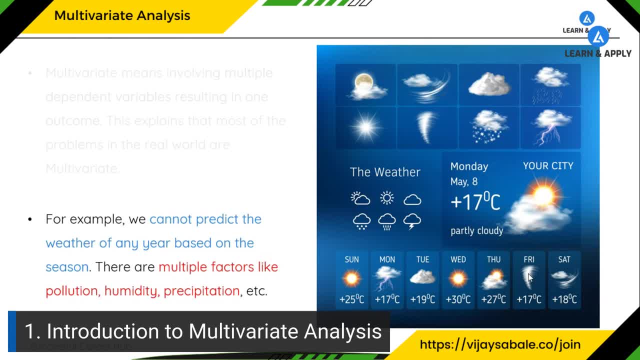 going to be the weather for particular year, right? So detecting the weather is not just depending on one or two factors, is the combination of many factors and we need to study all these factors so that we can predict the weather right. That's why it is the multivariate. Now, if you go into the 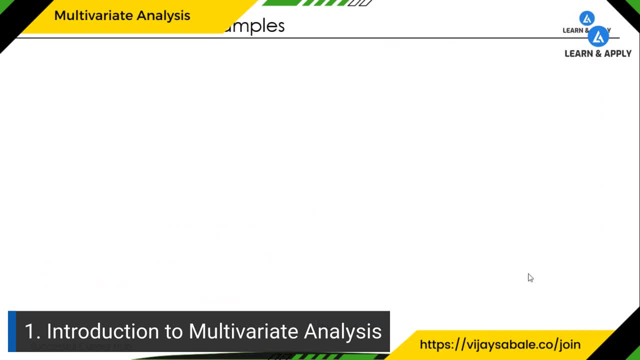 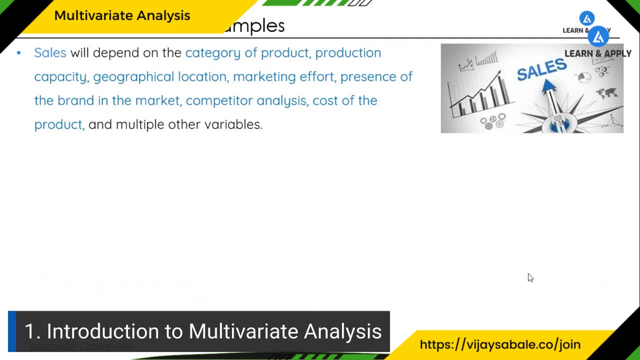 more detail to understand what are the practical scenarios. let's understand the sales- Sales of you take the any product or service you are going to sell. then it is again depending on the many facts, Like: what are the factors? is depending on the category of the product. It is depending on the 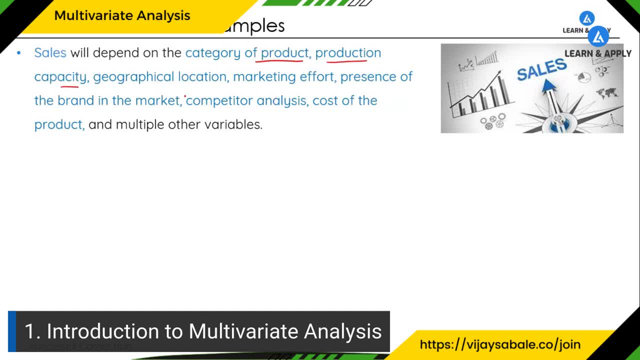 production capacity of that particular organization, particular plan, geographical location, marketing effort, presence of brand into the market, competitor analysis, cost of the product, and there are many number of factors on which the sale of that particular product or service is dependent. So we can see. if you want to study the sales, then again it's. 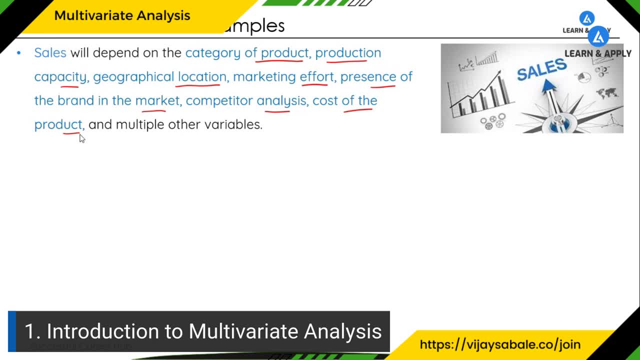 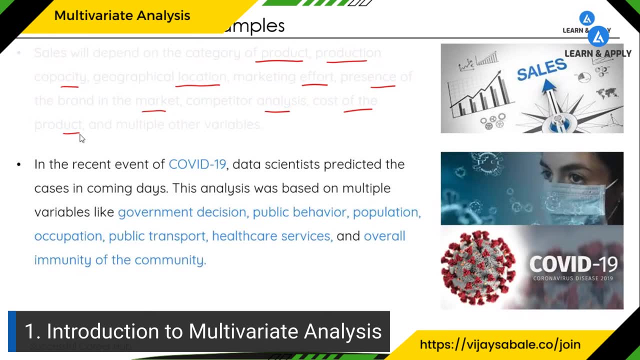 multivariate. We need to use the multivariate analysis. in that case, If you go into the more detailed examples, like if you go for the example of COVID-19, that was happened. we can see in the recent year of COVID-19, data scientists predicted the cases in coming days. 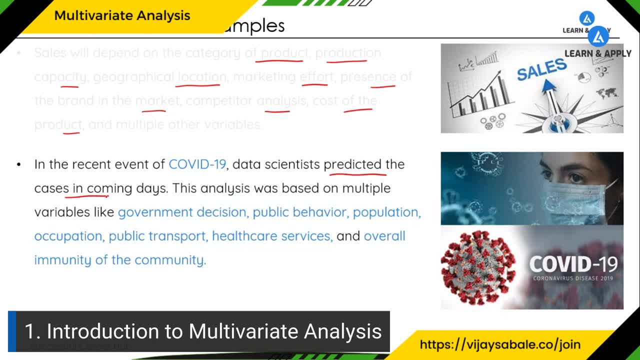 right Now how this prediction was happening. This prediction is again happening based on multiple factors. and what are these factors? These are the factors, but not limited to, like: government decision, governance, government policies, public behavior, population occupation, public transport. 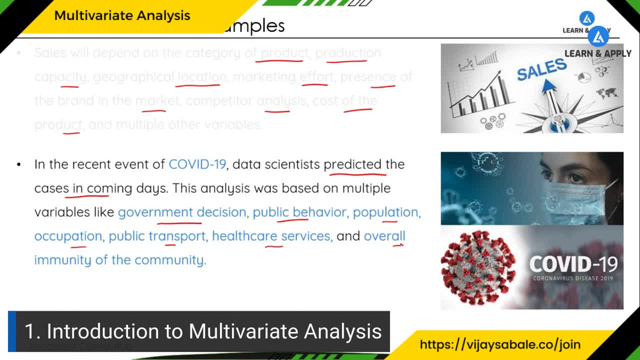 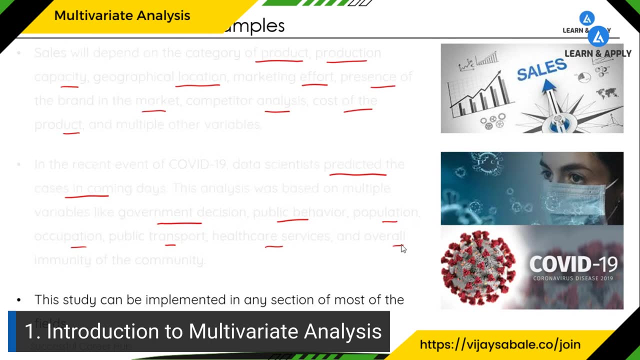 health care services and overall humanity of the community right. So it's a combination of many factors. In short, if you want to understand, this study can be implemented in any section of most of the fields and if you want to understand the many complex problems, in that case we need to use this multivariate analysis, these multivariate tools. So, in short, 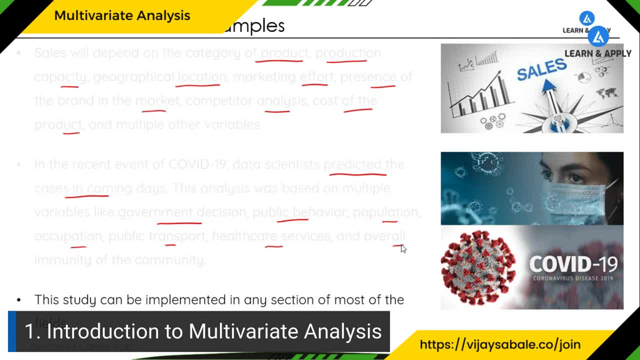 I can say: if you want to understand this multivariate analysis, you need to use this multivariate analysis. If you want to solve the problem that consists of the many number of factors, or the outcome, which has the combination of many dependent variables, in that case we must. 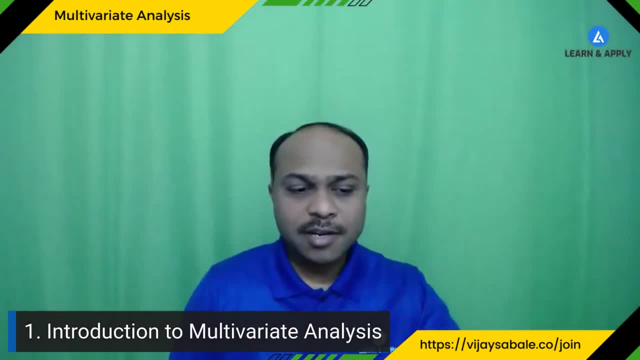 use this multivariate tools, right? Is this clear to you From the point in the discussion? I am sure that you must got the clarity about. okay, what is this multivariate analysis? at least, yes, Thank you so much, Monika. Thank you. Thank you so much, Atik. Okay, maybe your internet connection. please check, Atik. thank you so much. 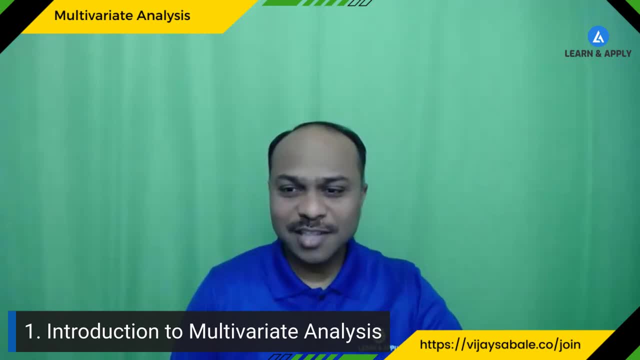 for your valuable comments. Please look into your connection as well. Thank you, thank you. Okay, so that's the importance of multivariate right. So there are many number of factors affecting our outcome. Now let's go into the second part, which is now: what are the terms that? 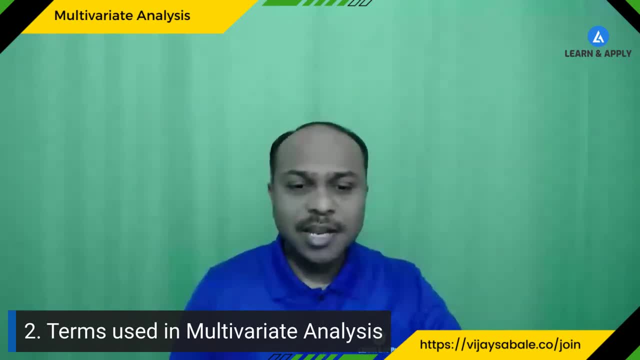 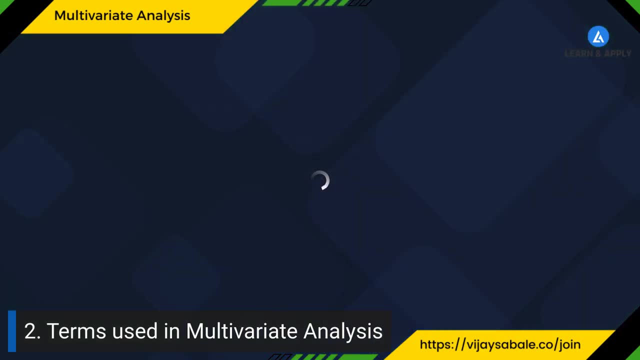 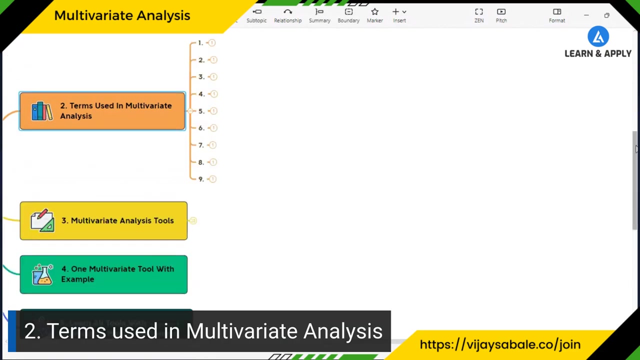 we need to understand before learning this multivariate analysis. So again, there is a huge number of important concepts that we need to learn. I have covered all them in detail in my training program, But just understand here what are these concepts? So here is a list of concepts that we 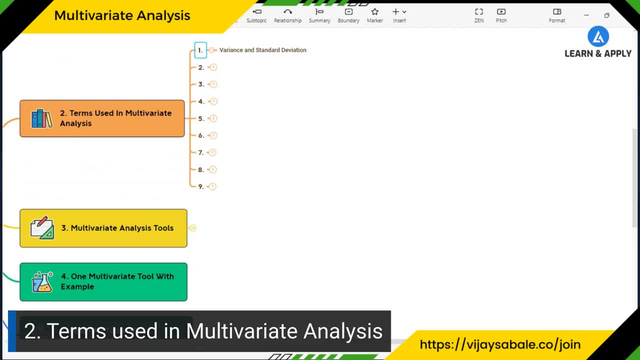 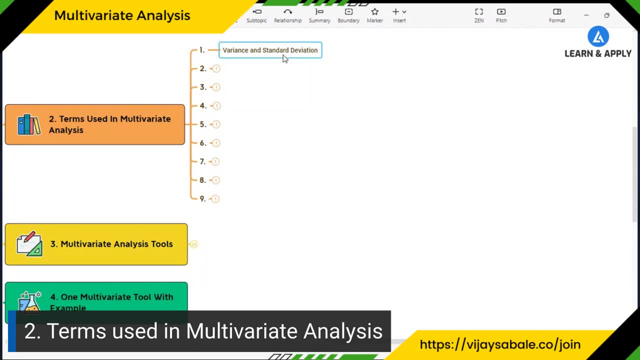 need to learn. The first concept is: we must know what is the variance and standard deviation. These are the metrics, these are the statistics which are indicating what is the standard or what is the variation into your data points overruns, eigenvalues and eigenvectors. These are, again, important concepts because 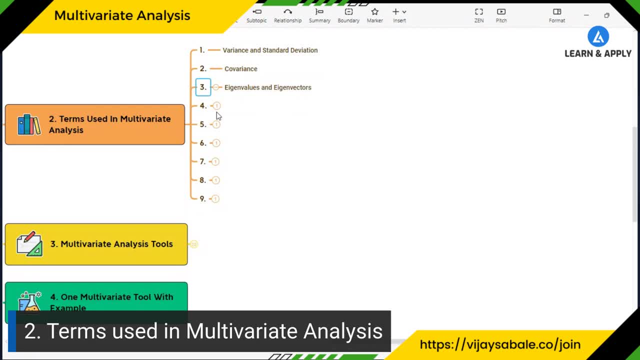 your interpretation of the results into the multivariate analysis is depending on these eigenvectors and eigenvalues. Then there is a principal components, factors. what is this meaning of principal components and factors? what is the dendrograms then? what are these graphs? 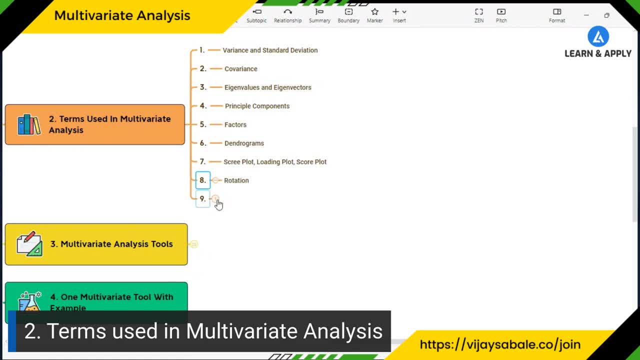 creep plot, loading plot and square plot. what are these rotations and what are the square coefficients? So there are many concepts and, as we are also going to take one of the example, I will explain some of the concepts into that. But if you have to learn in detail, it is really 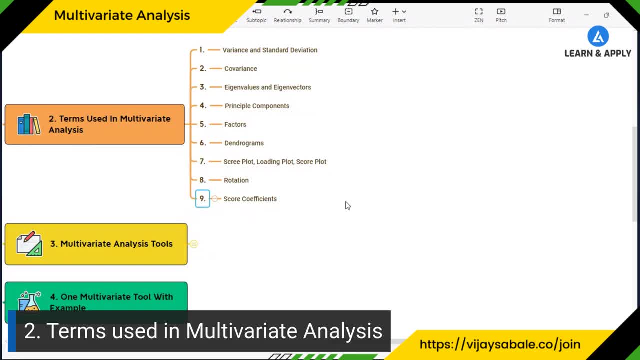 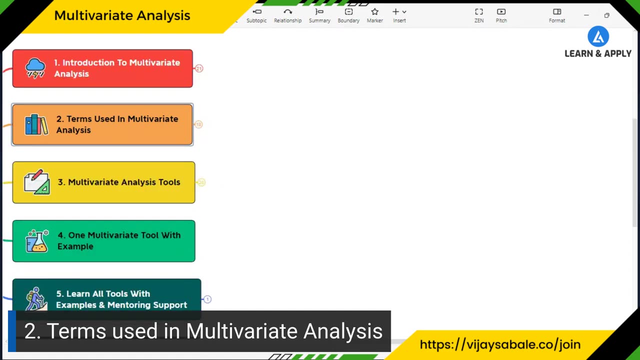 taking a time Due to time constraint. I am just explaining that as an overview. So these are the concepts that we need to learn. Anyway, as we are going to take the example, I will explain them. So these are the terms Till the point. do you have any questions? Please put into the. 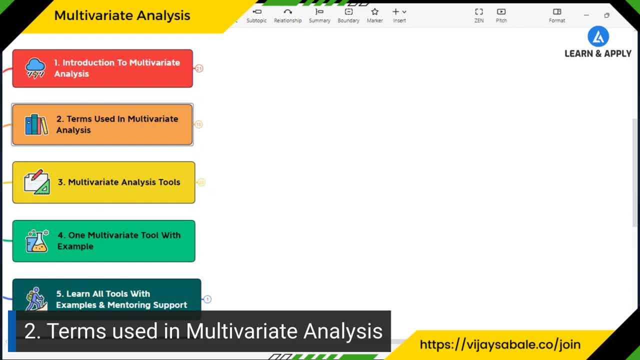 chat box so that I can answer your questions. Great, Thank you. So let us go to the third part, which is about multivariate analysis tools. Now we understood that: what is this multivariate, why multivariate analysis is important, why we need it. And then we had also seen, if you want, 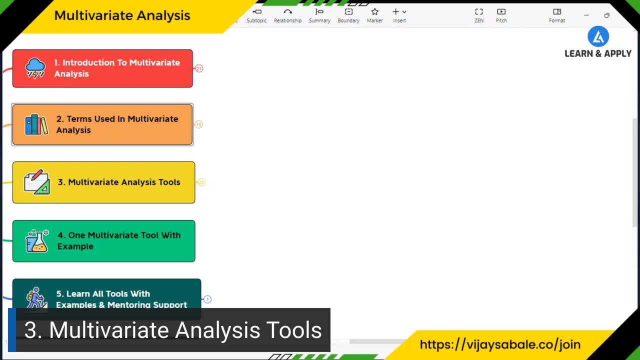 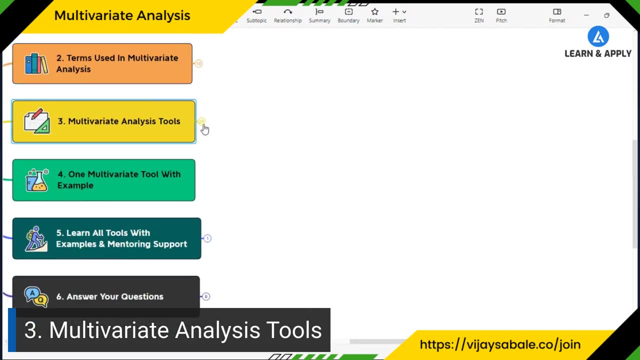 to learn this multivariate analysis, study of the some of the concepts is very necessary. Now let us go into the detail to understand what are these multivariate tools Or, when we are discussing about this multivariate tools, what are the tools it consists of, So we can categorize or 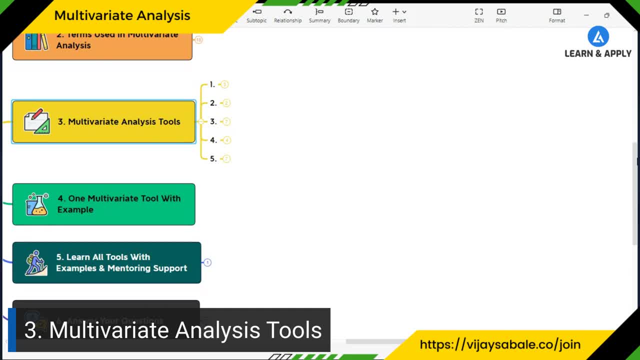 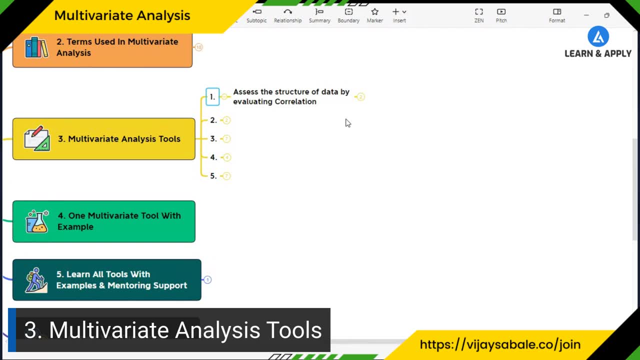 we can group them into five categories, or we can say there are five important groups of this multivariate analysis. The first one is: this is based on how we are going to assess the structure of data, by evaluating the correlation between variables. Let us say we are going to study. 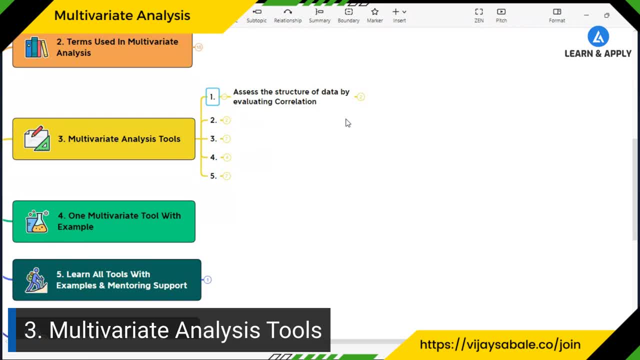 the 10 or 15 or 20 variables And if you are going to use the correlation between them to see what is the trend or what is the structure of the data. Now this is called as a assess the structure of data And that is done by evaluating the correlation between variables. Now this 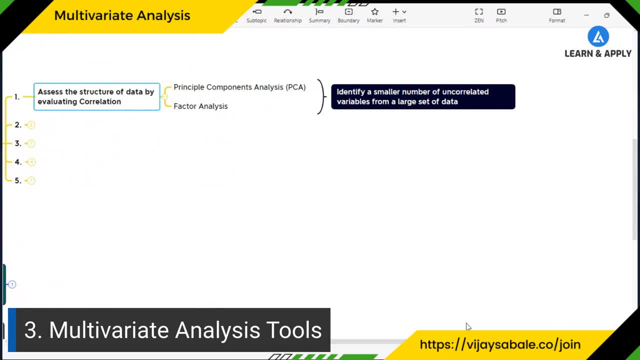 group consists of two important tools. The first tool is the principal component analysis And the second one is factor analysis. I am also going to explain this principal component analysis to you in the next class, Thank you. you in detail with the help of practical example, But let us understand here when we talk about. 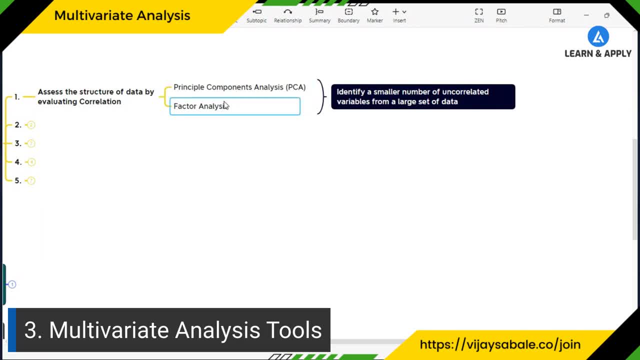 these two important tools: principal component analysis and factor analysis. actually, we identify a smaller number of uncorrelated variables from a last set of data. Right, let us say we are having the 10 or 15 variables From that. we are also from that entire variables. 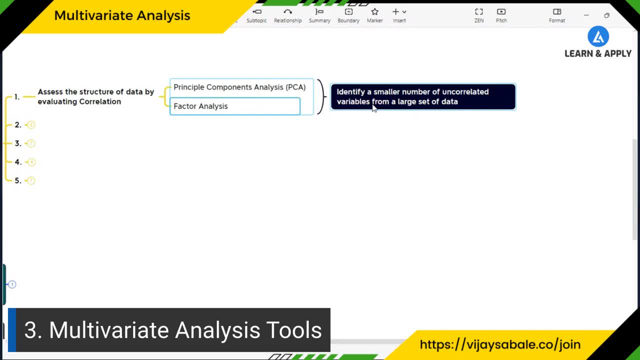 we are going to identify only two or three groups which are significant And we are going to name them so that we can have the better decisions Right. So, in principal, component analysis what we are going to do, we are going to convert the huge data into smaller number of. 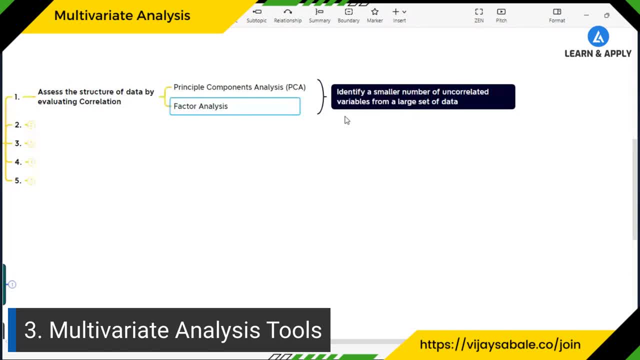 groups. These are also called as principal components or factors in case of factor analysis. Now, the second group is the item analysis. This is mainly dealing with these surveys. if you are having the data in terms of surveys, then we are going to use this item analysis. 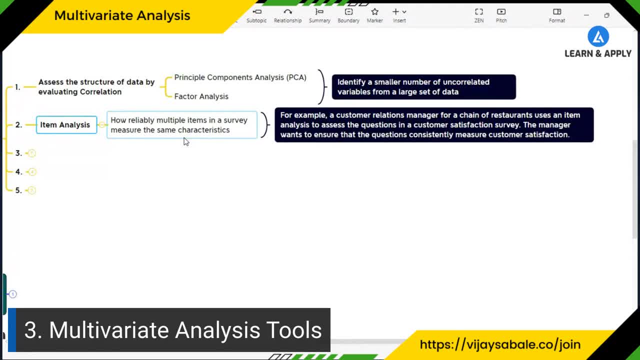 We can use this item analysis to see how reliably multiple items in a survey measures the same characteristics. For example, a customer relations manager for a chain of restaurants uses an item analysis to assess the questions in the customer satisfaction survey. In other words, we can say: 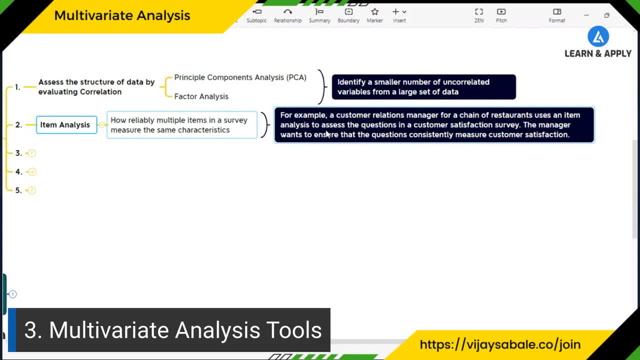 whether the survey that they are going to use to study the customer satisfaction survey, whether it is correct or not, or whether it is giving the significant results. The manager wants to ensure that the questions consistently measure the customer satisfaction, So that's a very important application of item analysis. Now let's go to the third part, which is 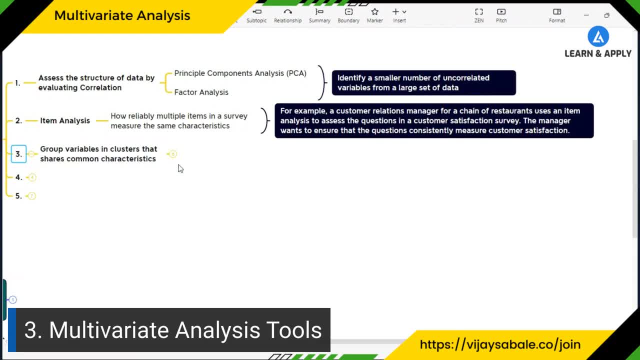 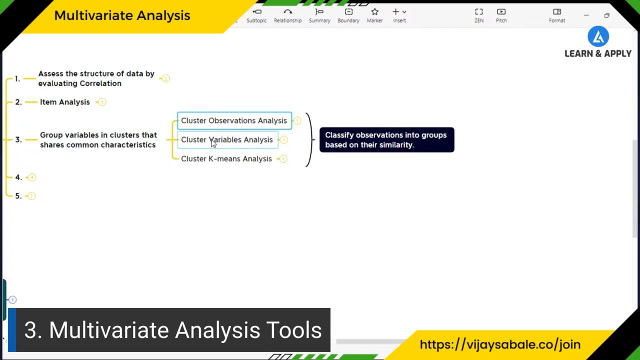 the grouping of variables and that is explained in terms of graphical results: Right Group variables in clusters that share common characteristics. Now, as a part of this, we are having three important types. The first one is cluster observations analysis. The second one is cluster variables analysis. And third one is cluster k-means analysis. 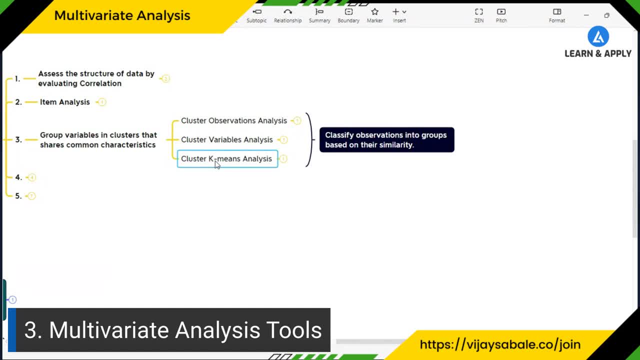 Here we are going to group the variables based on their similarities, Classify observations into groups based on their similarities. Now when to use which type? So there are some guidelines. For example, let's say, if you are having no prior information. 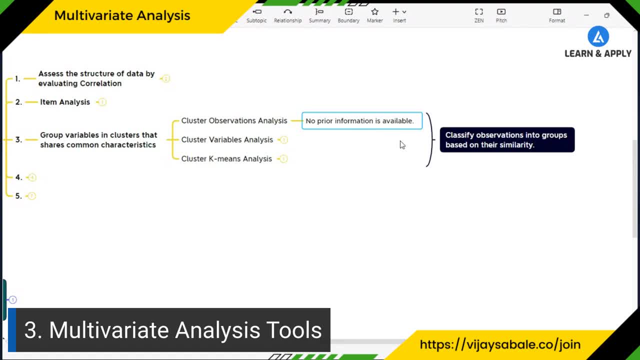 that means first time you got the data and you want to group them based on their similarities. In that case, we should use cluster observations analysis. Now let's say, if you're having some of the prior data available, that means we have some data and 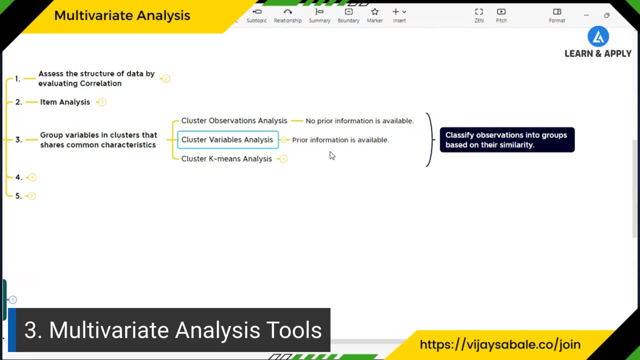 we know what is the background or what is the preliminary study that we have conducted into the history, then we can use cluster variables analysis In third part we are going to use when we are going to define how many number of groups that we are going to form Right. 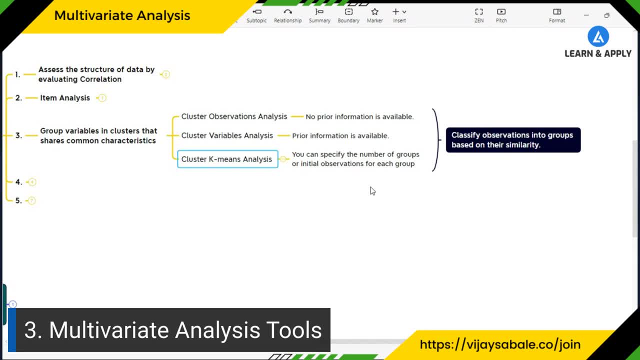 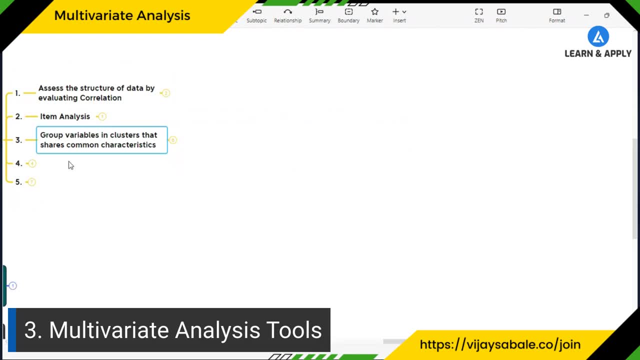 You can specify the number of groups or initial observations for each group. Then in that case we can use cluster k-means analysis. This is the third group. Now the fourth group is about discriminant analysis. In many cases we are going to see that, yes, there are processes are capable. 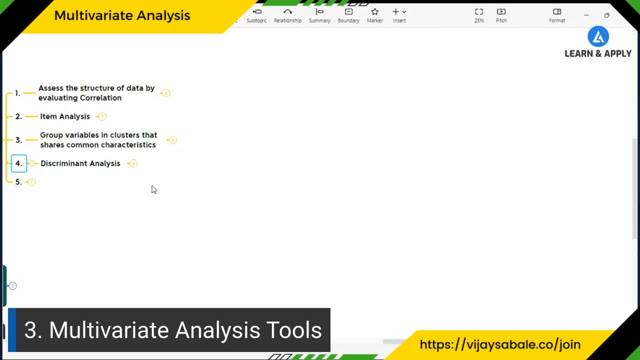 but still we are getting some defectives and it's really hard to detect what is the root cause for it. The investigation and everything is getting more time, required, more time, And in that case we required some immediate actions. Discriminant analysis is a very powerful tool that we can use. 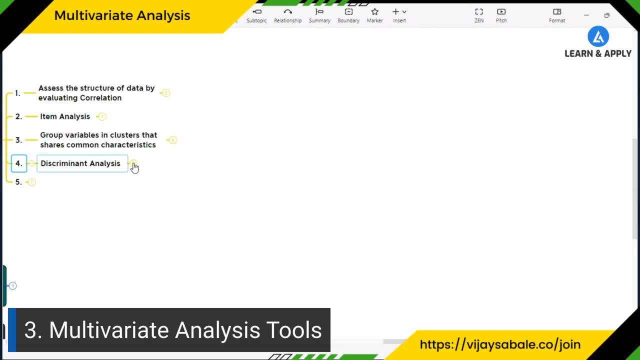 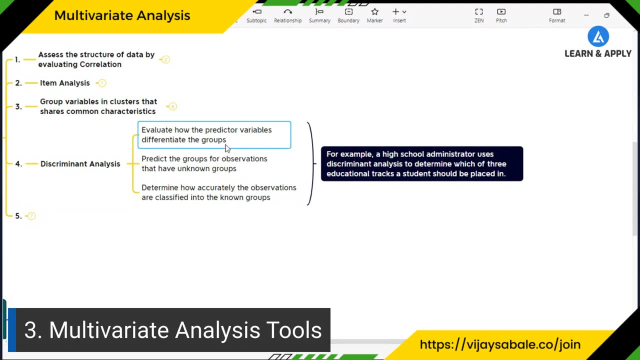 In such situations. now, what are these situations? for example, to evaluate how the predictor variables differentiate the curves. Let's say we want to talk about the defectives and non defectives. Right, So how we can define the particular product of particular services, defective or not? 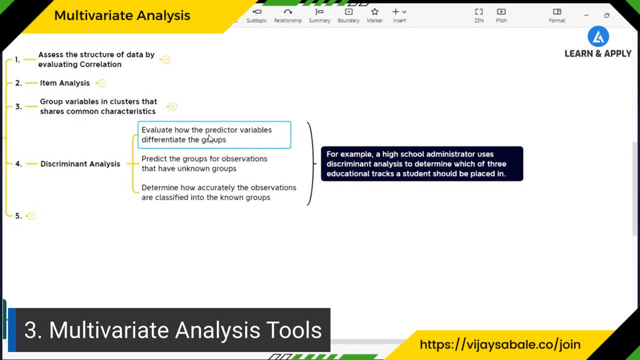 In that case we are going to use the discriminant analysis. Evaluate how the predictor variables differentiate. Second: predict the groups of observations that have unknown groups. predict the groups for observations that have unknown groups. that means if you got the observations, we must know in which category or which group it belongs. determine how. 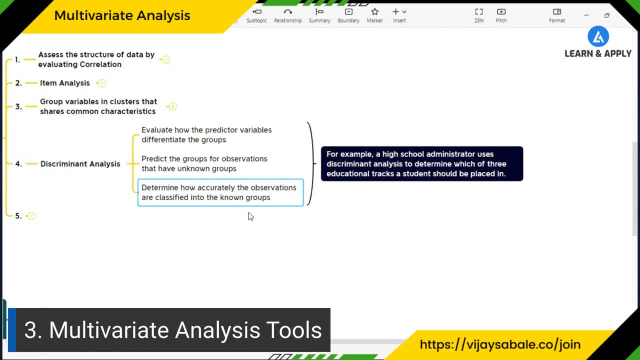 accurately. the observations are classified into the known groups. so we can also check the accuracy. depending on the eigenvalues that we are getting, we can say, okay, which is the most suitable group, that but group for that particular observation right. so again, this is a very powerful tool. 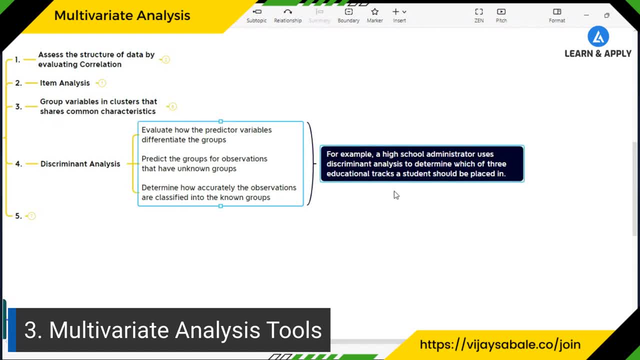 and here is an example. for example, a high school administrator uses diskament analysis to determine which of the three educational tracks a student should be placed in. so there are three educational tracks like a, b, c, a is like the students who did not require any attention from the teacher. 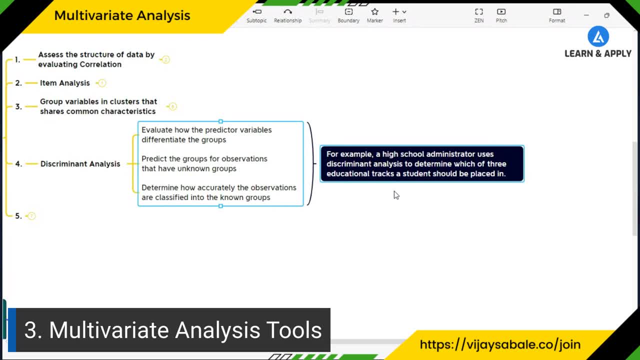 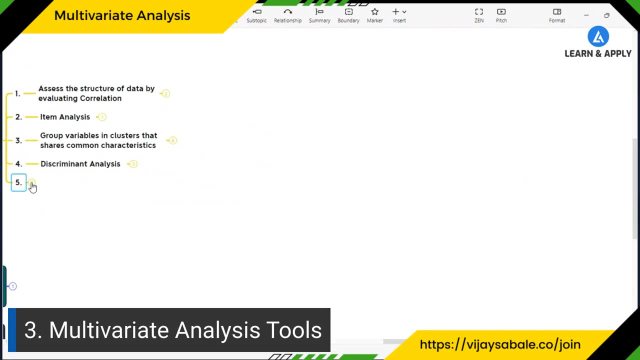 b, because some attention is required. and c- yes, very high attention is required from the teachers. and to group the students um, um into these three categories, we can use the discriminant analysis. This is again very powerful tool. And the fifth group of these multivariate tools is called as correspondence. 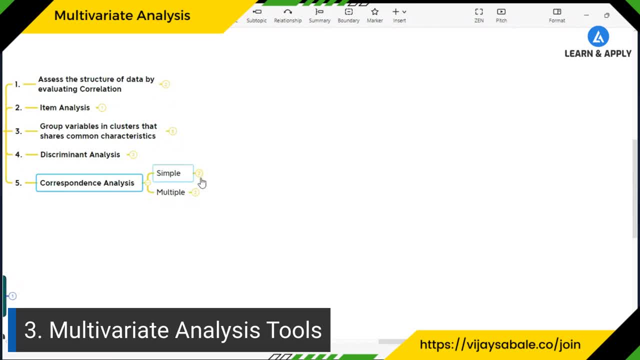 analysis. Now, what is the application of this? Correspondence analysis is used to understand the relationship between many variables and to group them for easy analysis. These are having the mainly two types. The first one is called as a simple and multiple, As the name indicates. 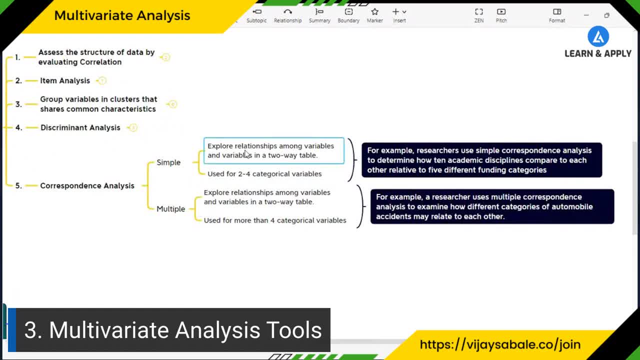 simple and multiple. we can see here Simple analysis, explore the relationship among variables, and variables are in a two-way table. Now what is meant by two-way table? There is a one-way. The table is having the two dimensions. One is the one variable and the second is having the 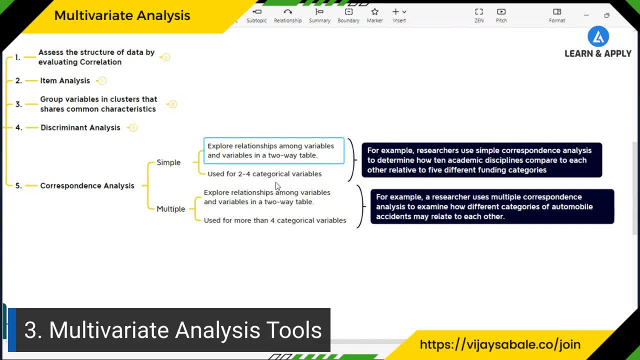 another variable. We are going to use up to two to four variables. If you're having two to four categorical variables, then we are going to use simple correspondence analysis. For example, a researcher use simple correspondence analysis to determine how 10 academic disciplines 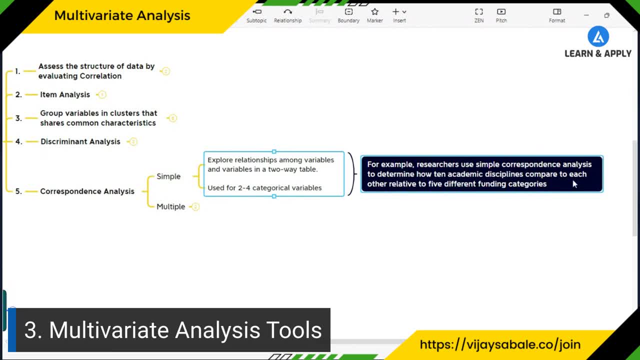 right Now, academic discipline is a one variable to each other, related to five different funding categories. So the funding category is another variable. So we are going to see the relationship between these two categorical variables having their multiple elements, right In that case? 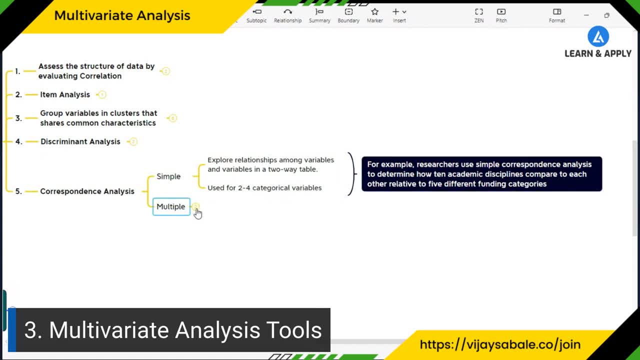 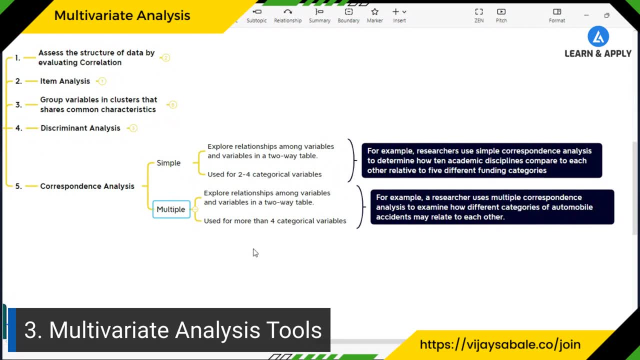 we are going to use simple correspondence analysis. Now, application of the multiple correspondence analysis is nothing but the multiplication of the simple correspondence analysis. This we are going to use if you are having the more than four categorical variables. Application, if you see it is the same, Explore relationship among the variables and also the data. 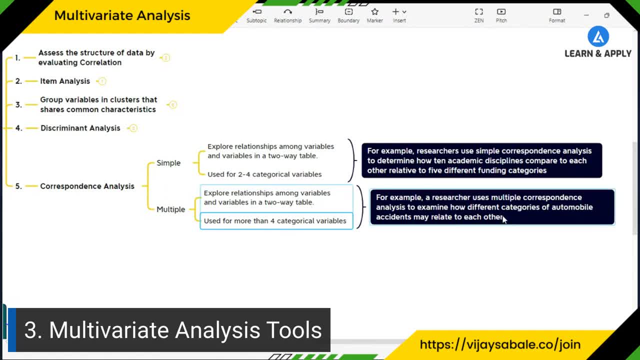 is in two-way table. For example, a researcher use multiple correspondence analysis to examine how different categories of the automobile accidents may relate to each other. So here we have number of combinations, many number of groups that we are going to study here, right And in that. 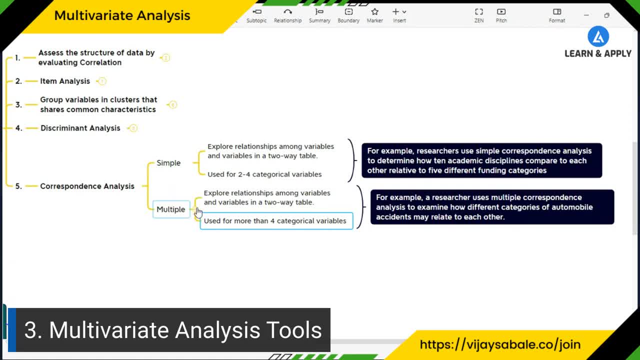 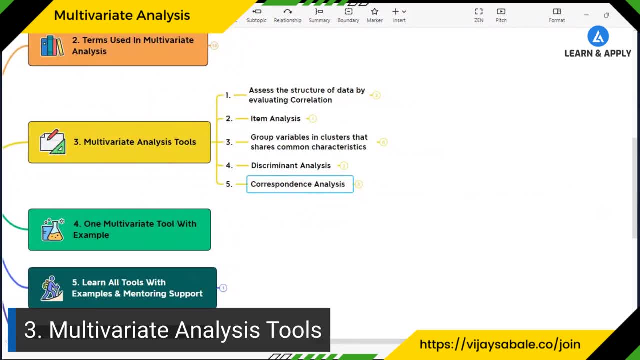 situation. multiple correspondence analysis is the most important tool, right. So these are the five important groups. In my training program, I have explained each and every topic in a very detail with help of practical examples. So these are the five important tools, five important groups that 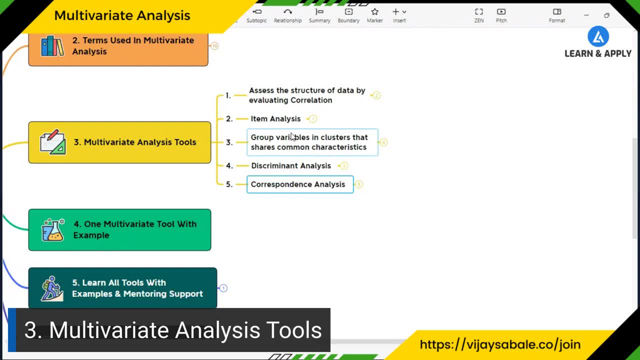 we are going to study, as a part of this, multivariate analysis tools. okay, Do you have any questions? Still the point: Okay, great, No questions, Great. So let us go to the fourth part, which is we are going to learn one multivariate tool with the help of example. okay, So let me share with 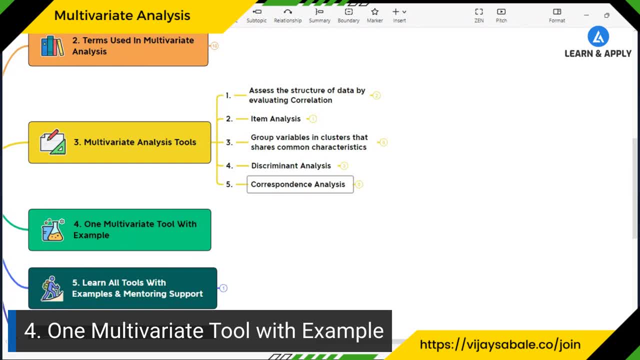 the screen and let us learn that. I am also going to demonstrate you how we can perform that into the Minitab, so that you can also learn how to perform that into the Minitab. So let us go to the fourth part and let us also have the understanding of it. So let me share the screen. 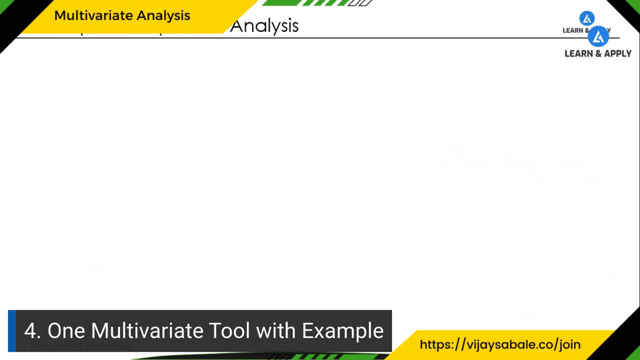 So the tool that I am going to explain is a principal component analysis. Now, what is the application of this? As the name indicates, principal components. so we are going to convert, we are going to identify, we are going to group the variables. 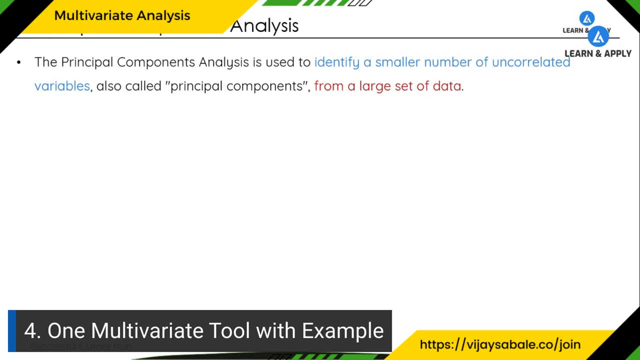 in such a way that we can have the maximum number of variation into same or smaller number of variables. The principal component analysis is used to identify a smaller number of uncorrelated variables, also called as principal components, from a last set of data. With this analysis, 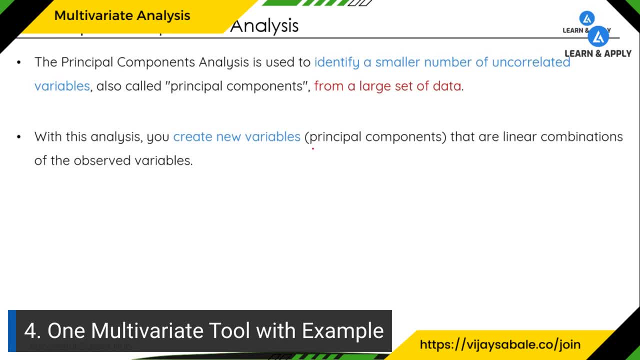 you create new variables. Now these variables are also called as principal components. So we are having the new group of variables, and these are nothing but the linear combinations of the variables that we have observed or that we are using for the multivariate analysis. 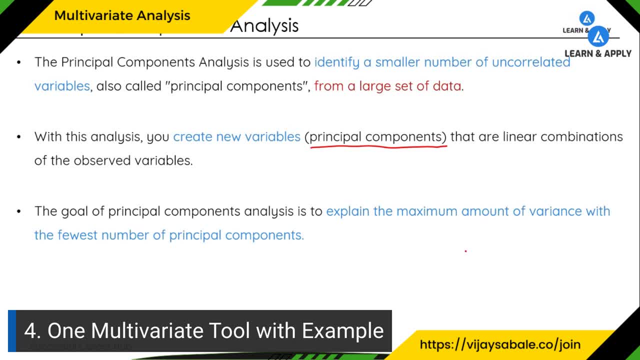 The goal of principal component analysis is to explain maximum amount of variance with the fewest number of principal components, and that is why this is very powerful. Let us take an example so that we have the clarity about how much powerful this principal component analysis is. 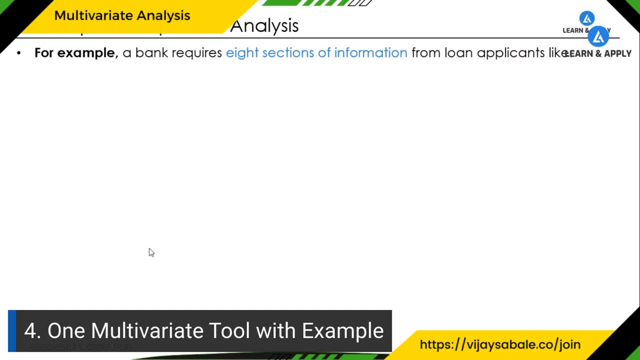 For example, a bank requires eight sections of information from loan applicant right. So this information consists of: what is the income of that person, what is the education age, residence time, work experience, savings, debt and how many credit cards that person. 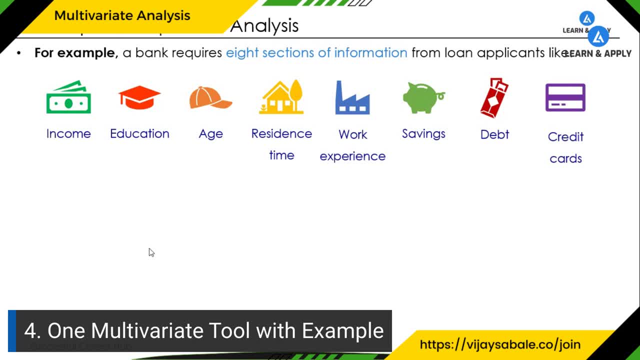 is using right. Based on these eight factors, the bank is going to decide whether they are going to give the loan for that particular person or not, right? The bank administrator wants to analyze this data to determine the best way to group and report it right? So we are going to group all these eight variables into the principal. 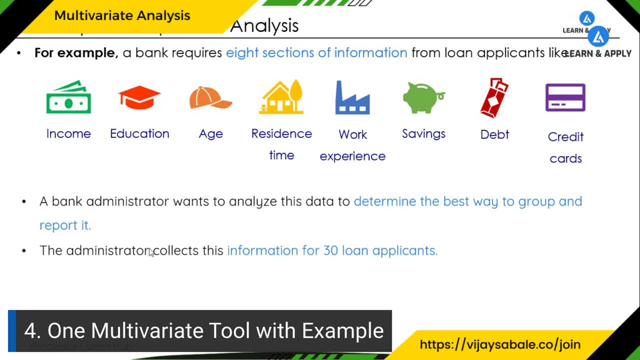 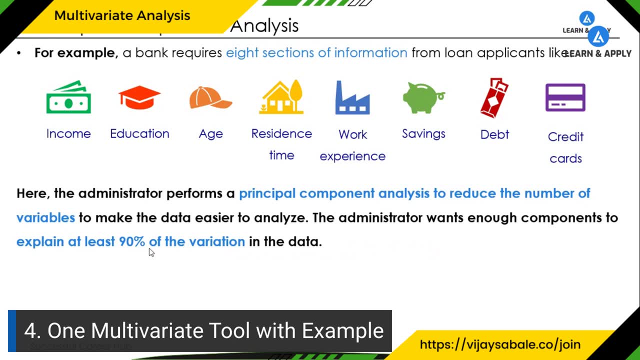 components that will make the bank to take decisions very easily. The administrator collects this information for 30 loan applicants. right Here the administrator performs a principal component analysis to reduce the number of variables. as we are having the eight number of variables, Can we reduce it to the one or two? 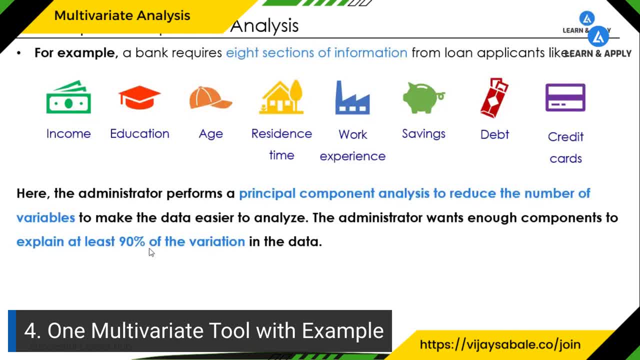 Two or three So that we can have the minimum number of variables to take a decisions. The administrator wants enough components and how much? At least they should explain 90% of variation into the data right, And that's why we are going to use this principal. 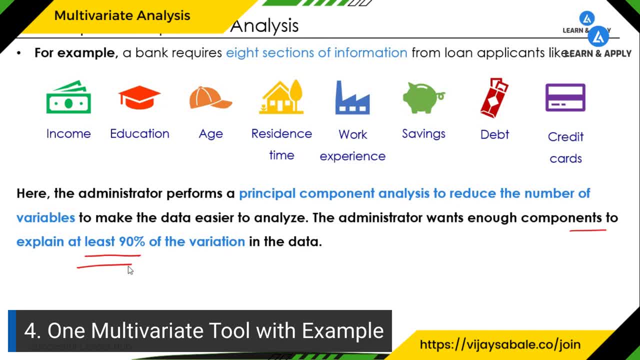 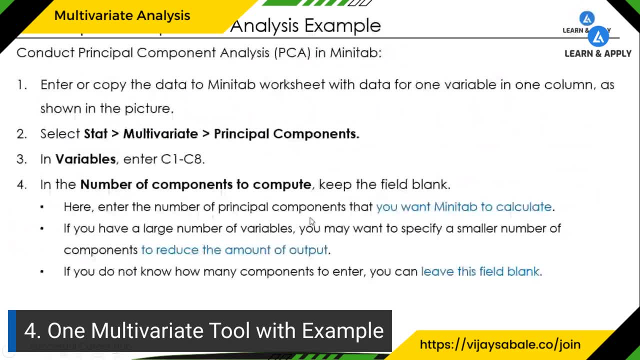 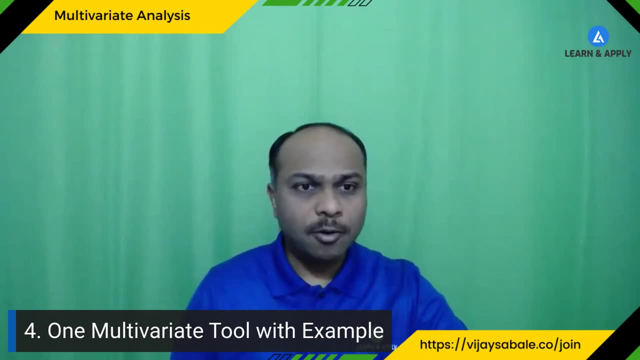 component analysis, How we need to follow to perform this principal component analysis. So let me share with that data and how we can perform that into the Minitab. So that's it. You can also have the more clarity on that, okay, So let me show you the screen. 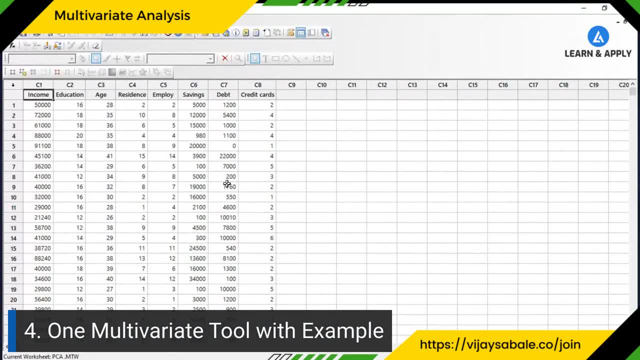 Okay, can you see my screen? This is the Minitab worksheet and which has the data for all these 30 applicants for these eight variables. So this is the Minitab worksheet and which has the data for all these 30 applicants for. 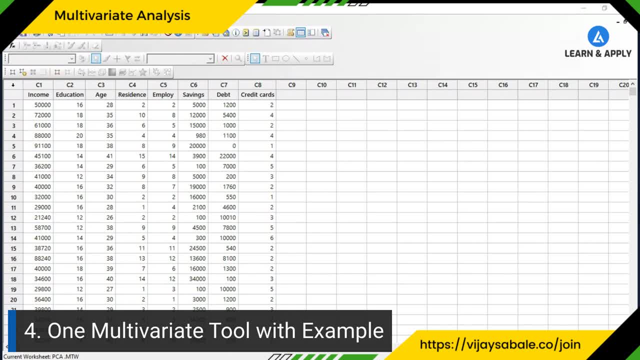 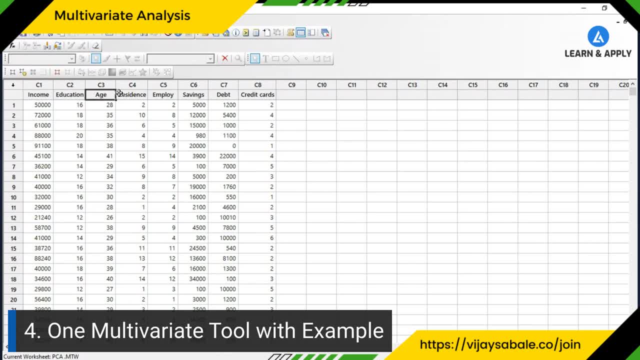 So let me show you the screen. We have eight variables, We have a list of eight factors. eight variables, right? So let's go into the detail of it. It consists of the income, education, age, residence, how much? duration of the employment. 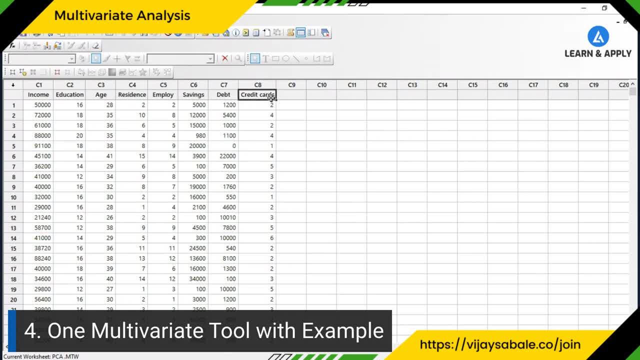 savings debts and how many number of credit cards that applicant is using, and this data is collected for 30 loan applicants right And now. instead of all these eight variables, eight factors, we want to group them as per their similarities so that we can have the decision making process. 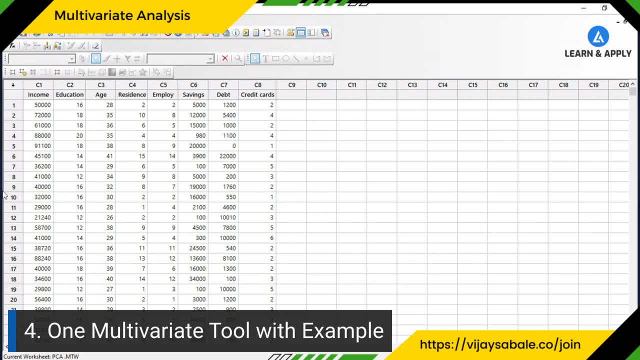 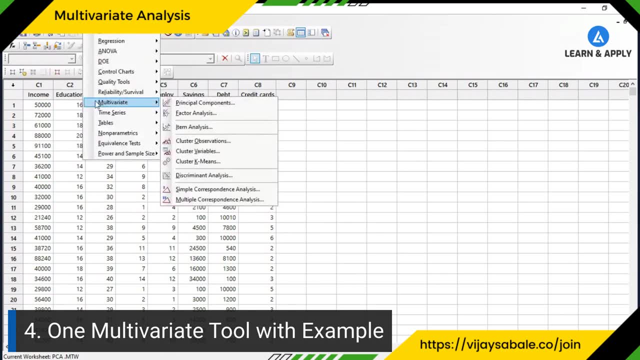 making very easy to pass the loan right. so let's perform this principal component analysis on this data go to the stat. then we need to select this multivariate options and after that we can select both of these options. we can also use the principal components or factor analysis, application of both. 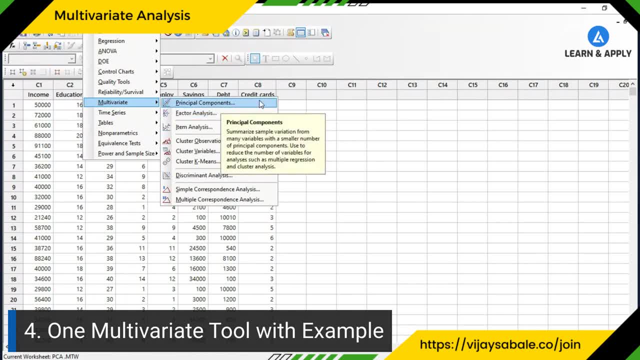 of these is a very same. now let's talk about the principal components. summarize sample variation from many variables with a smaller number of principal components. in short, we are going to group all these eight factors, eight variables, into smaller number of groups, so that our decision will be much easier used to reduce the number of variables for analysis, such as multiple regression. 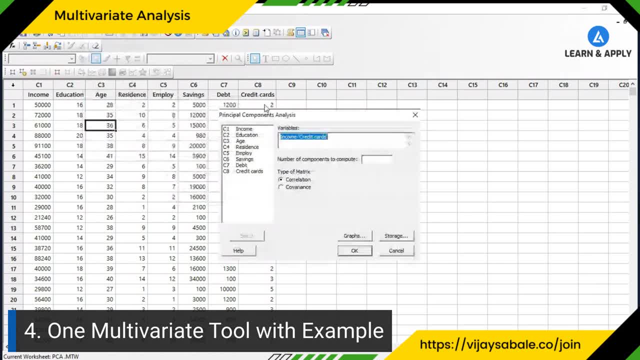 and cluster analysis. so click on that. now, here we can see we need to provide some data like how many number of variables that we are going to study. let's say, we are going to study the number of variables that we are going to study and we are going to study the number of variables. 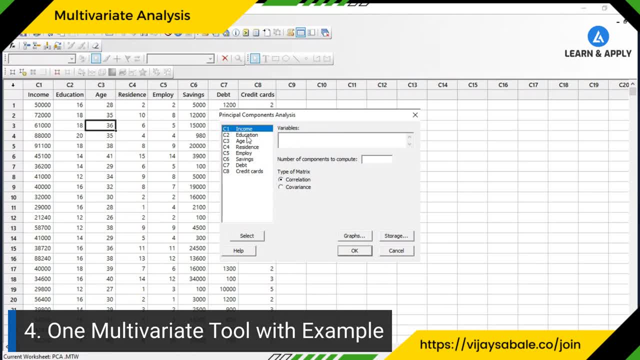 all these eight variables to select. so select all these eight. income to credit cards: select. that means we are going to study all these eight factors. number of components to compute: we can insert here any number or we can keep it as a blank so that minitab calculate based on their. 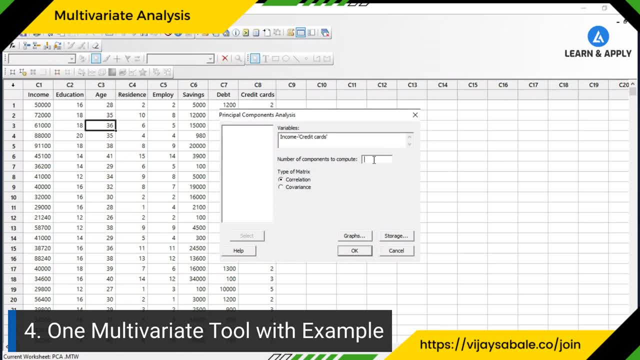 feasibility, right. so at this point of time let's keep it as a blank. and there is a type of matrix. so there are two types of matrix. the first one is called as a correlation and second one is called as a covariance. correlation type of matrix is used when scale of the variables is 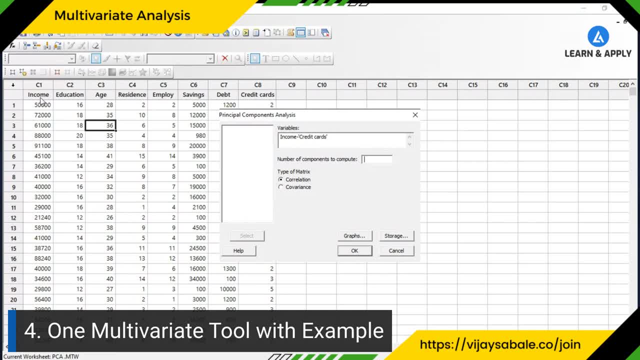 different. for example, if you see our data income, for the income scale is different, like we can see, the minimum value we are getting here is around 20, apresent to 40, and higher value is coming around. 是啊, something around ninety one thousand hundred. right, so there is a huge cell. 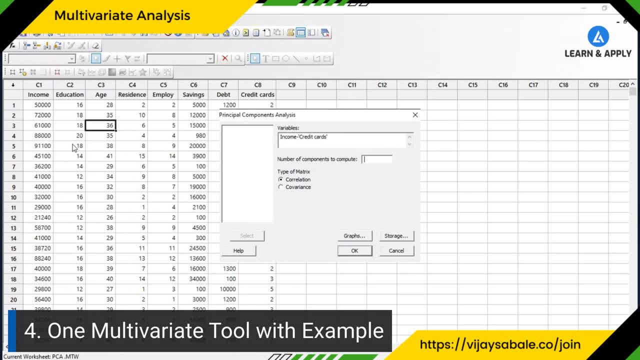 huge scale and if you have to compare that with irrespective of the education scale, again it's a different value that we need to flying the random variable and that's that's why it is useful at the different scale, because we are having 12 to 20 something scale. for age, again there is a different. 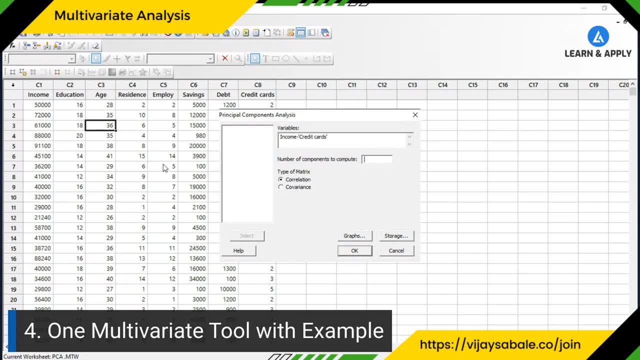 scale. residence- different scale. employee number of years for the employment- again different scale. savings- again there is a another type of scale. so we can see the scale for all the factors, all the variables that we are going to study, is not same, so we need to select this correlation. 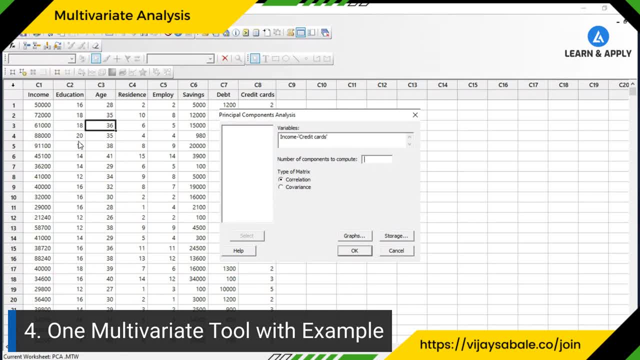 type of matrix. if you are going to use the same scale like 1 to 10, right, in that case we need to use covariance. if you click on the graph, there are five graphs are available, like screen plot, score plot, loading plot and by plot for first two components and there is outlier plot once we plot. 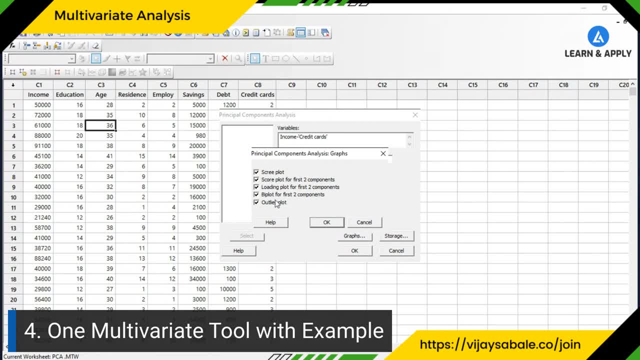 these. i will also explain what is the meaning of them and how we can input the results. okay, at this point of time, let's select all these graphs, click ok, that's it, so that that is the input that we need to provide to the minute app. once we provide that input, click. 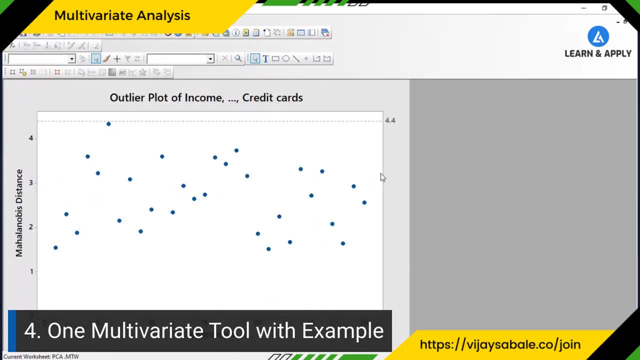 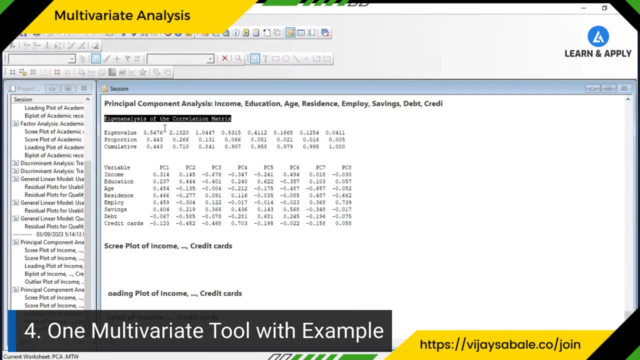 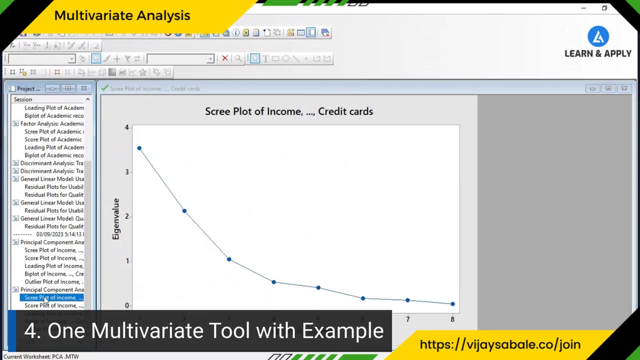 on. ok, so that we will get the output. now, if you go into the detail, let's see what are the output we are getting. we got the one eigenvalue of the correlation matrix, then we called all these principal components and after that we got these five graphs when a scree plot, then score plot. 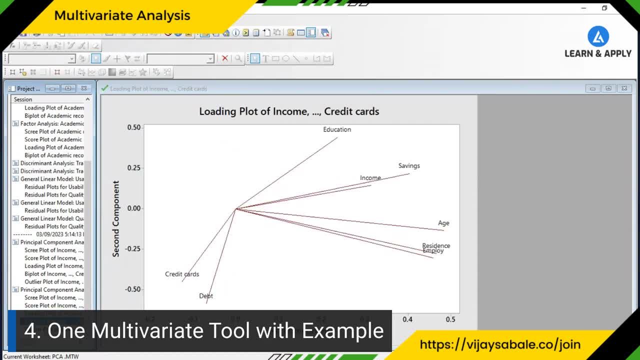 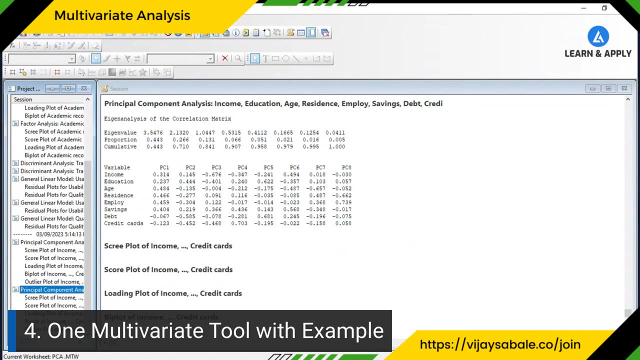 loading plot by plot. and the last one: there is a outlier plot. okay, so let's go into the detail. I explain: what is the meaning of all these, the matrix that we had seen, and what is the interpretation of this graph. what is the meaning of them? okay, so let's go into the detail of it till the time do. 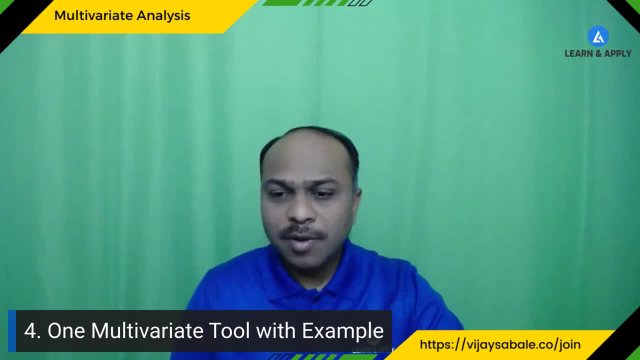 you have any questions? is dendrogram multivariate tools? dendrogram is coming as an outcome of the cluster observation analysis, so we can say it. the outcome that it gives it is like the how we are going to group the number of variables right, so it is going. it's a very beautiful graph and it also explained like. 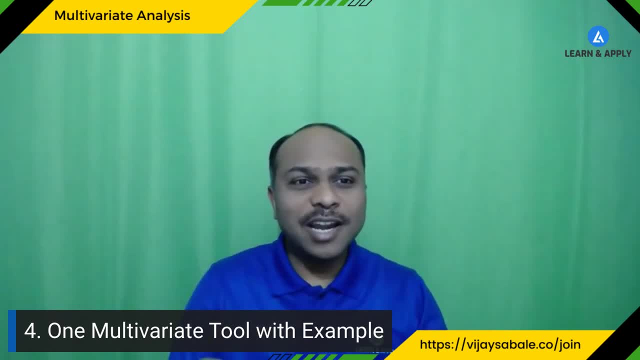 the we can talk about the family tree. it is going to indicate which variables are belong to which category. right, that's a really great tool. thank you so much, Carlos, for asking this question. great, thank you. okay, now let me share with the outcome into the presentation and we have some discussion. 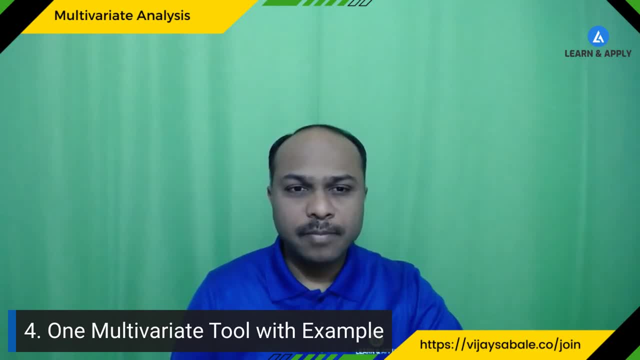 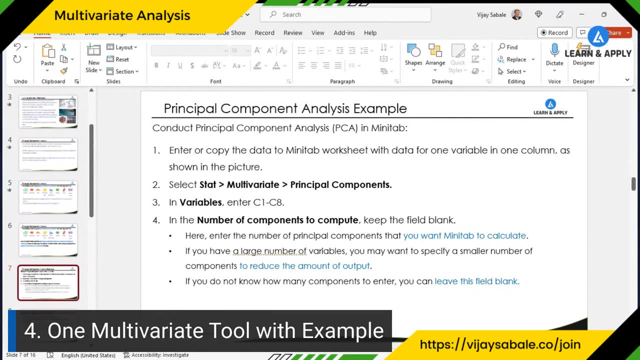 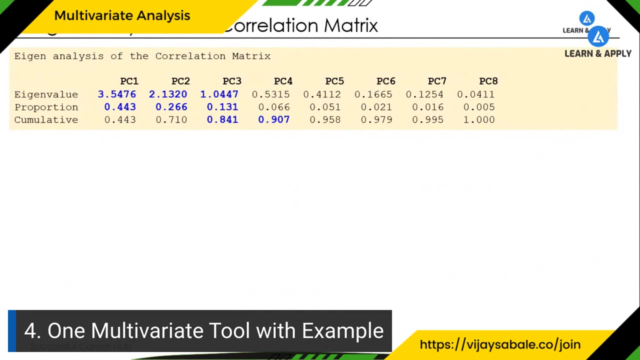 on that. okay, so we have seen this. yes, so this is the first correlation matrix that we got as the first outcome from the analysis. right, and here we can see what it consists of. it consists of all the principal components. so PC, nothing but the principal components, and we got all these principal components. 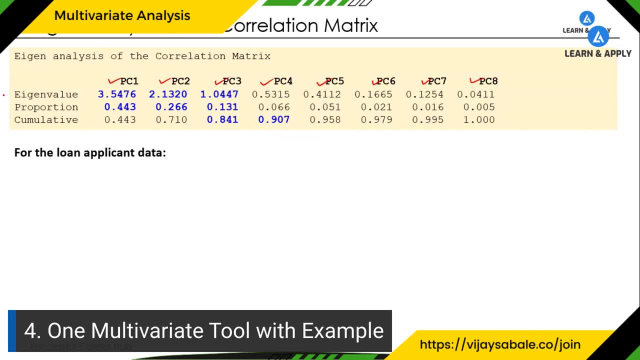 now, if you see here, the first row is eigenvalue and also that how much cumulative percentage. now, if you talk about the principal component one, it indicates the eigenvalue as 3.5476. now what is this indicates? this indicates the variance. this indicates the variance. so we can see the 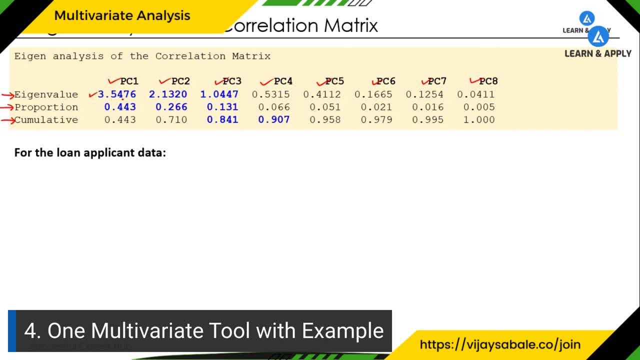 first principal components has the huge variance or the highest variance compared to the other things. and if you see the, what is the contribution of this principal component? one is a 44.3 percentage. so this first principal component is having the highest voltage that we can see. it's a 44.3 percentage of the contribution into 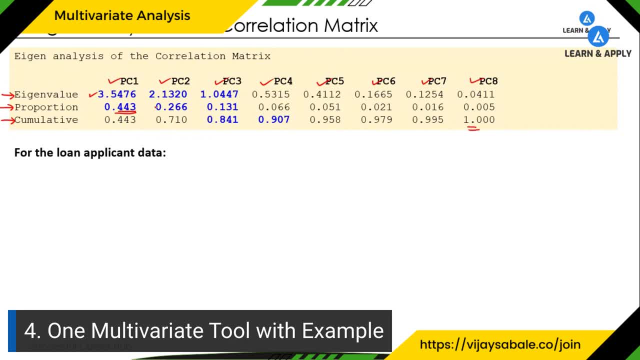 overall 100 of the variance, right? so we need to focus on this principal component one. if you go to the principal component two, its contribution is- two point sorry- 26.6 percentage. its contribution is 26.6 percentage and has a value for variance, or the eigenvalue is 2.1320 if you add the principal component one and two together. 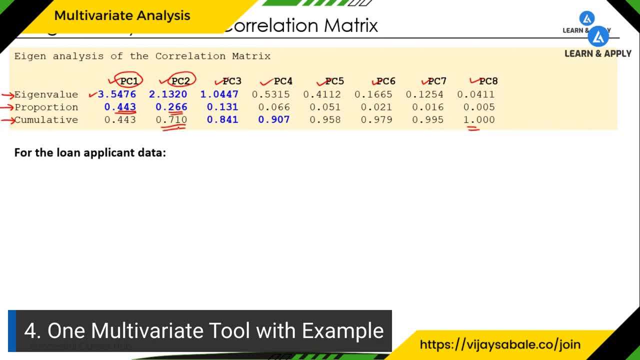 they are contributing 71 percentage. have we calculated this 71 percentage? 44.3 plus 26.6, so that is coming as 71.. if you look at the principal component three again, it has the eigenvalue of 1.0. four, four, seven and its contribution is thirteen point one if you add principal component one, two. 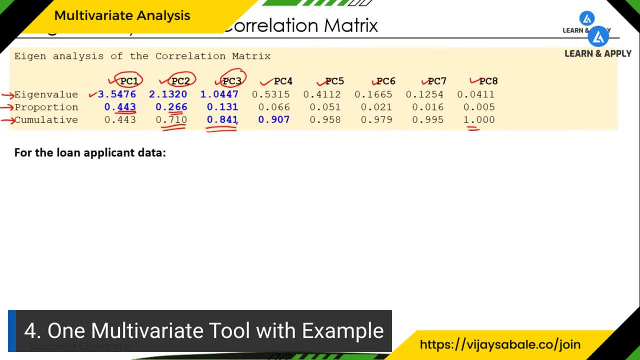 and three, so all three come together explains 84.1 percentage of the variation. if you add the fourth component again, it explains 6.6 percentage, and if you add all these four it explains 90.7 percentage. now, if you go back to the example, the administrator wants to see how many number of principal components. 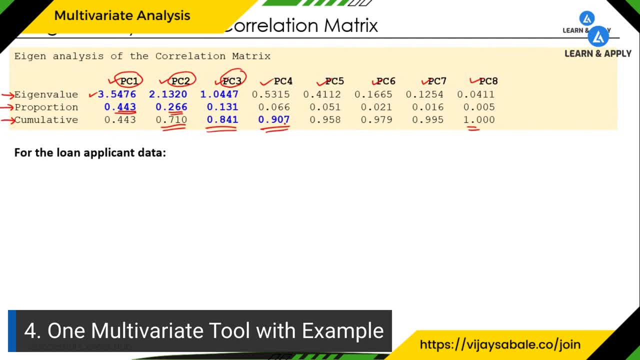 that will explain 90 percentage of the data, right? so here we can look for or we can take a data after the four principal components so that they are going to explain 90 percentage of the data, right? so this is the interpretation of this correlation matrix. this is the same thing that I have explained, the first principal component. 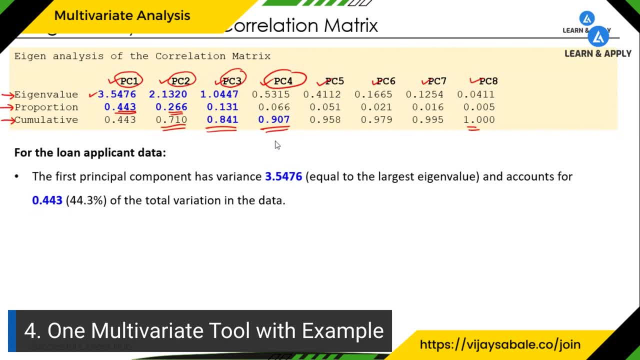 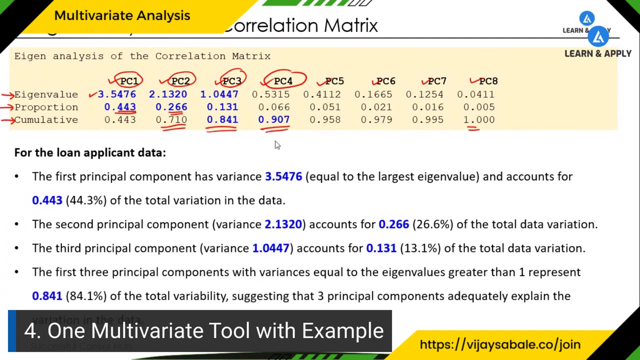 has variance of 3.5476. that accounts for 44.3 percentage. second is 26.6 percent, with the value of two point one. three third, thirteen point one percent, with the value of one point zero four. and then there is a fourth component. if you add the first three component, they are explaining 84.1. 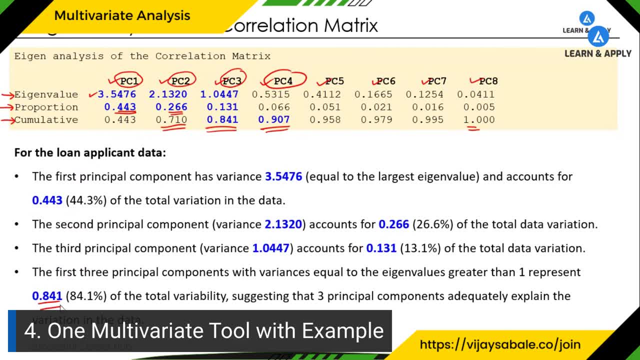 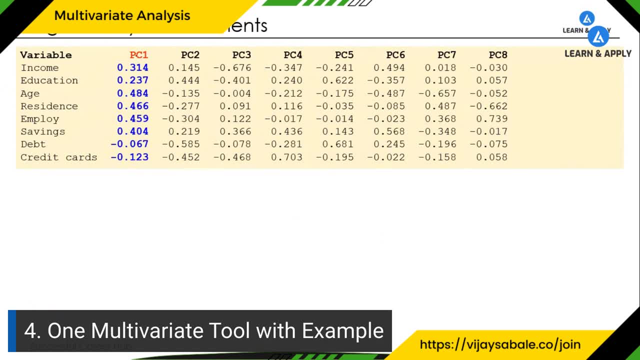 percentage of the variability out of 100 percentage. now let's go for the eigen analysis coefficients. now, if you see this principal component one and the variable, then what it indicates. it indicates what is the value of this principal component one and how it is calculated by, because these are also. 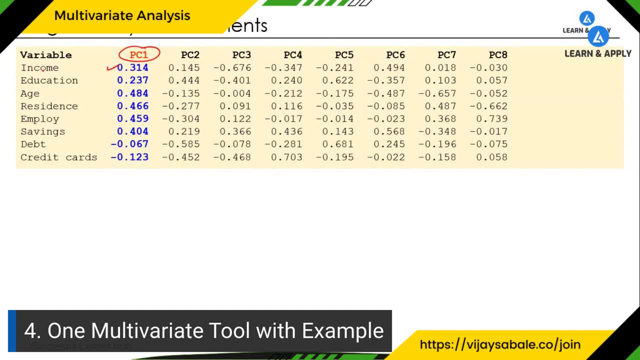 considered as a coefficients. so if you multiply this coefficient with that particular value of that variable, then we will get the first element of this principal component one. in short, if you want to calculate the principal component one, value that can be calculated by the coefficient of the income multiplied by the value of the income, right? so the fixed equation will be like: 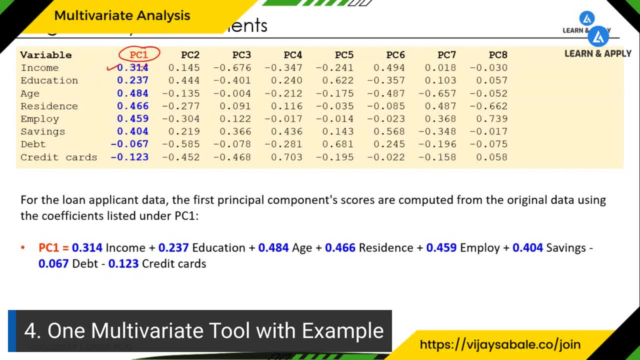 this: 0.314, that's the coefficient for this principal component, one multiplied by the income, 0.237 multiplied by education, plus 0.484 multiplied by h, 0.466 multiplied by residence, and in similar ways, right here it is a minus, so we can also see the values coming as minus minus 0.067 into. 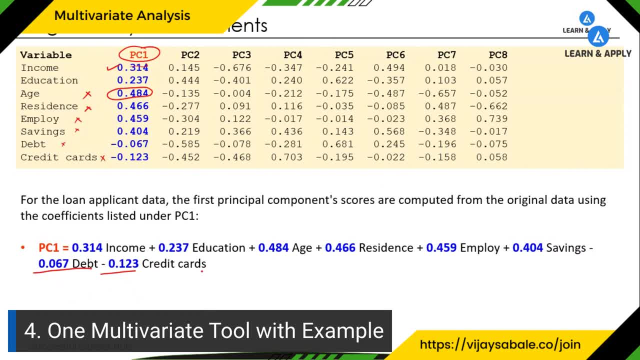 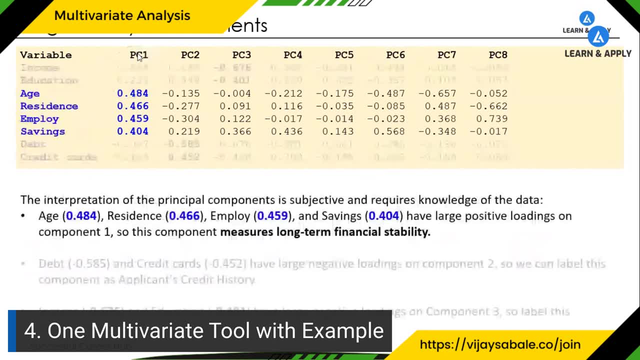 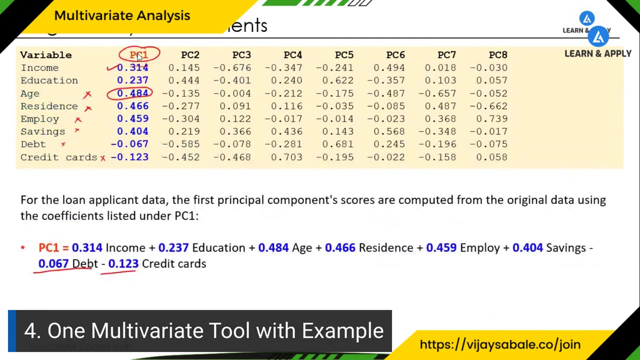 tech and minus 0.123 into credit cards. right, by using this coefficients, we can calculate what is the value for the principal component 1. similarly, we can also calculate for that principal component 2, 3, 4 and so on. now, the intent of these values, this coefficient, is that we are going to group. 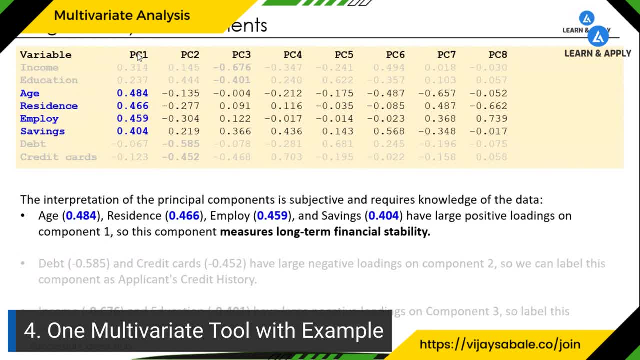 them as per their values. now, if you look at the four variables of the four coefficient here- for the age, residence, employer and savings, all are having the about the same value. that is point 4, 8, 0.46, 0.45 and 0.40. right, so the values are very close to one another. that indicates that they form. 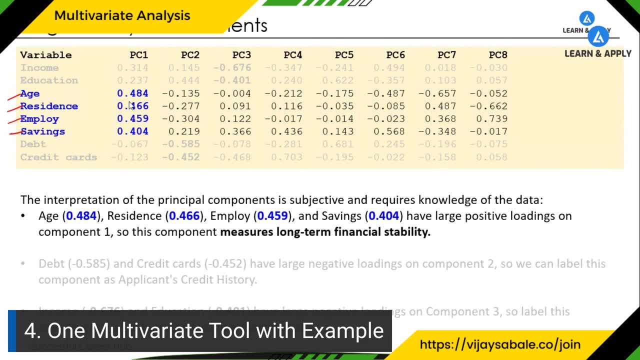 the one group, right? so based on this coefficient value, we are going to group them. now, if you go to the second principal component, we can see this: depth and credit cards has the same value around minus 0.58 and minus 0.45, so we can group them as a second group. and if you go for the 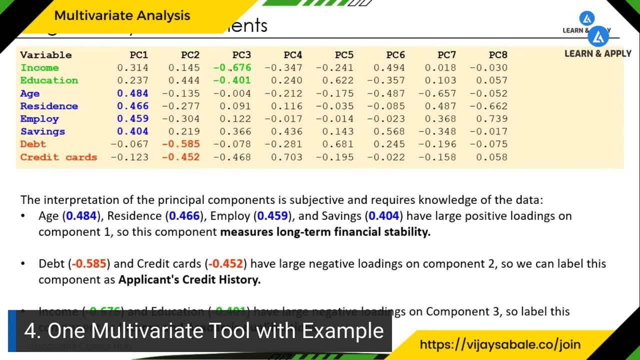 third principal component. again, we can see these two values minus 0.676 and minus 0.401. we can group them into the third principal component. now again, if you can see, here is a minus 0.468. these values again close to this, but as we have already considered the credit card into the principal. 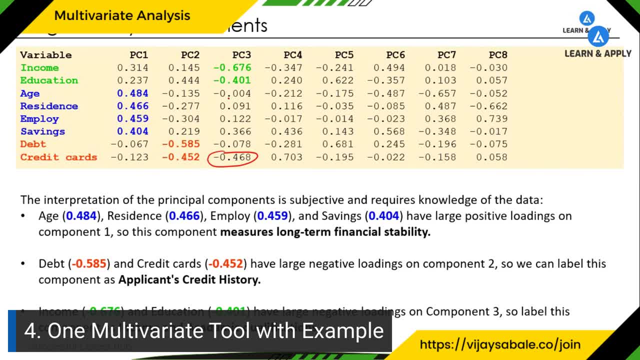 component 2: let's talk about the another variable, and that is the education here. so if you consider these two variables- income, education- we can predict or we can have the third group, which is called as a principal, component three. Now, once we group them, we can name them as per their similarities. 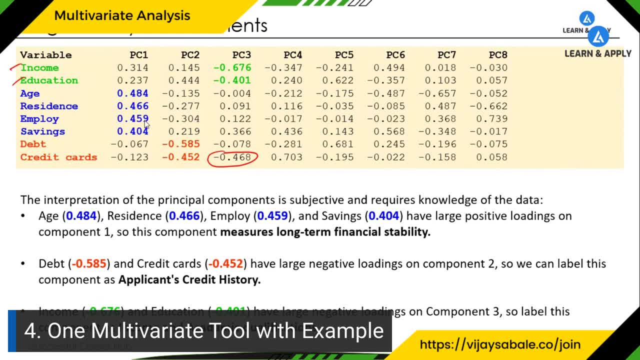 Please remember that we must have the subject matter expertise, subject matter knowledge, so that we can group them. For example, if you talk about the first principal component, that consists of the age, residence employee and savings that can be termed as a long term financial stability. 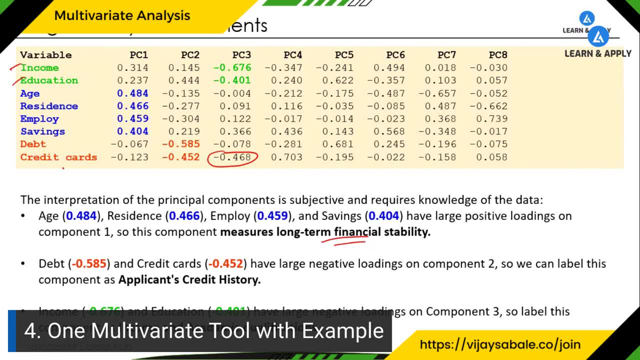 The second principal component, debt and credit card. they can be grouped as applicant credit history. And the third principal component, income and education. that can be called as an income and academic qualifications right. That means if the bank administrator wants to issue or wants to pass the loan for the 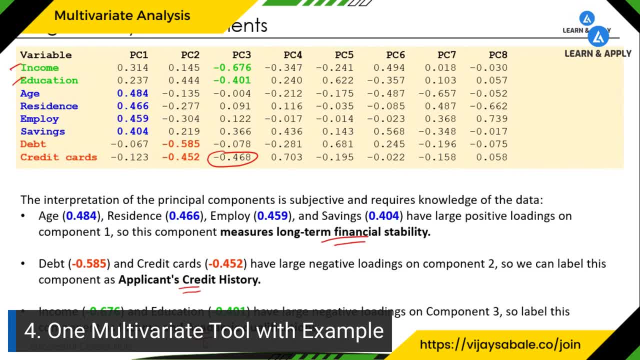 particular loan applicant, then he should only focus on three variables. The first one is what is his or her long term financial stability, What is his or her credit history And what is the income and academic qualifications. That means, instead of focusing on the eight variables, now they are grouped into three. 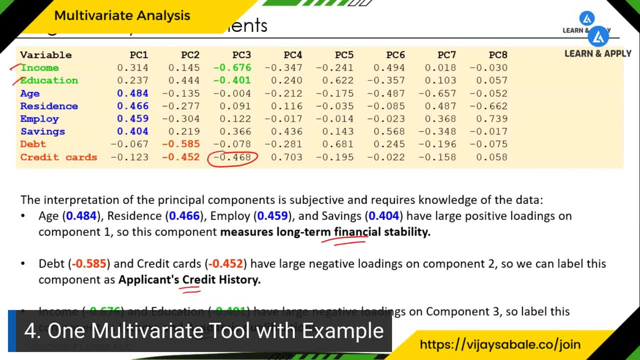 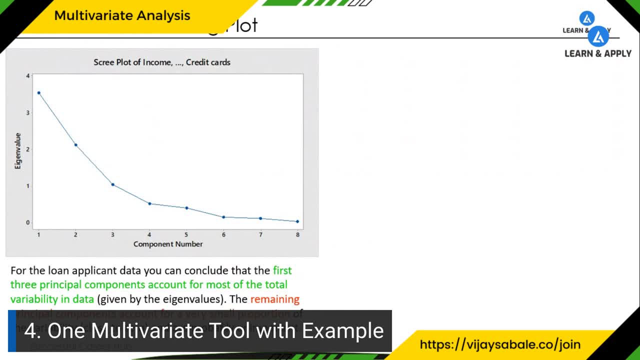 principal components as per their similarities. So this is the power of this principal component analysis. Now, if you see how much important of each of these principal component that is indicated by the screen plot, So we can see there are eight principal components: One, two, eight. 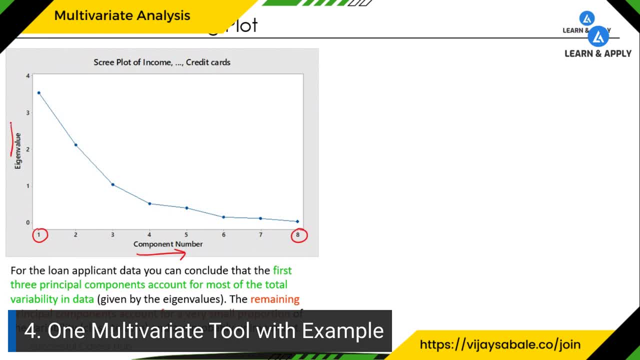 You can see here and there is eigenvalue, And it is always a pattern that first principal component has the highest value of the eigenvalue. Second principal component has the next eigenvalue compared to the principal component one, and so on, And it is going to be deteriorated or it is going to be reduced. 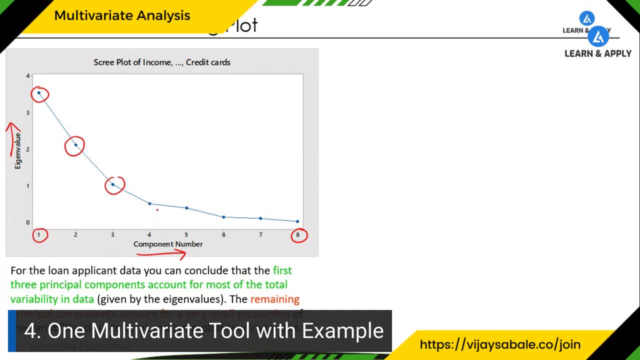 We need to decide up to which value we should interested or we should look for. For example, if you go up to the fourth principal component, Okay, Okay, Okay, Okay, Okay, We are getting around 90 percentage of the variation. 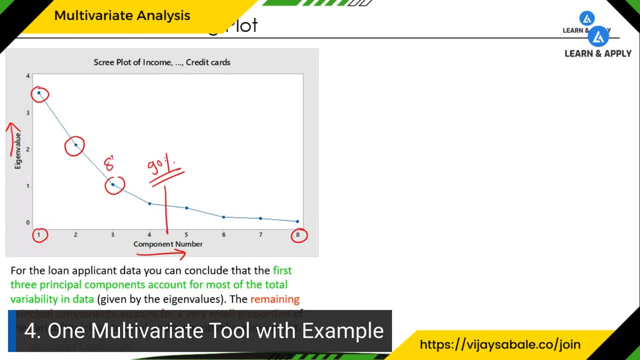 Or if you end up up to the third principal components, that is also okay, because we are having the 84 percentage of the data Right. So we should focus, or we should only consider how many number of principal components based on what are the reasons that we want? 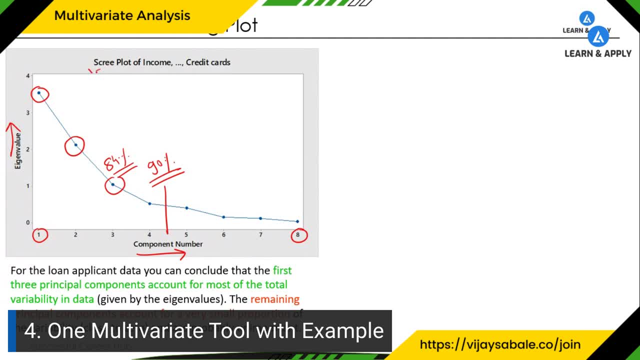 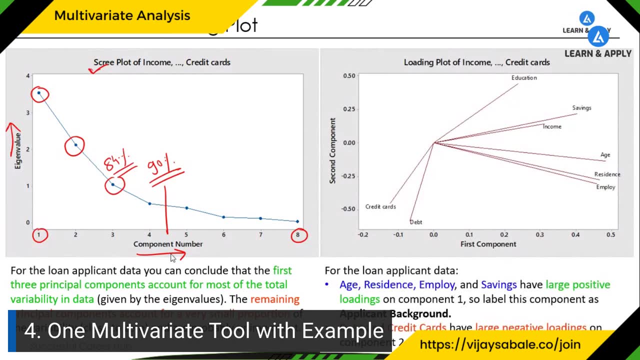 Okay, So this is the screen plot. Screen plot indicates distribution of the eigenvalue with respect to principal components. Now there is a second plot, Which is called as a loading plot, In that, the loading plot, the by plot and the next plot that we are going to see score. 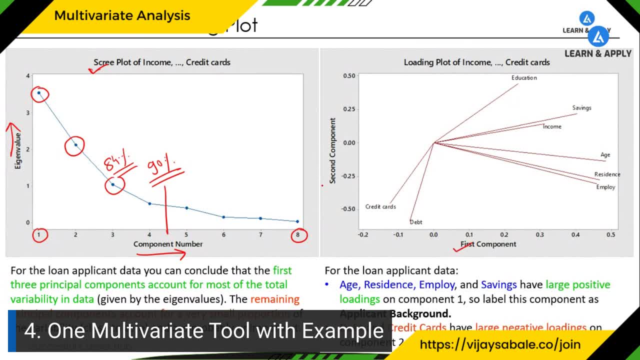 plot that are only for the first two components, And why it is so? because we have seen only the first two components are having the highest importance compared to the other principal components. So, instead of focusing all the principal components, we can just focus on first two: one and two. 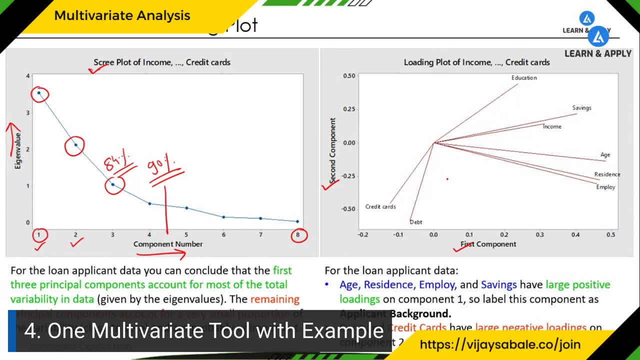 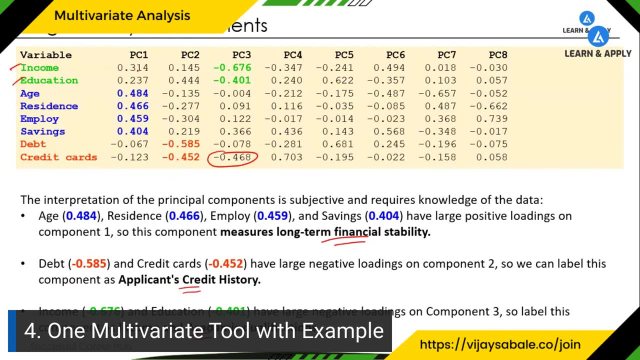 so that we can have the more results. Now, if you see the values of that coefficients that we had seen Here like principal components, the income is 0.314 and for principal component two is 0.14.. So if you use these two value as an coordinates, like X coordinate and Y coordinate, then we 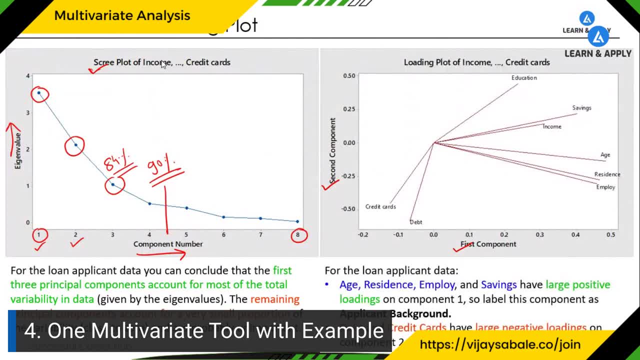 are getting one point into this graph on the loading plot Right. And similar way, if you plot all these eight variables onto this loading plot, we are getting the different lengths for each of the variables. Now the length These variables are having. if you compare these similar lengths, they are going to be grouped. 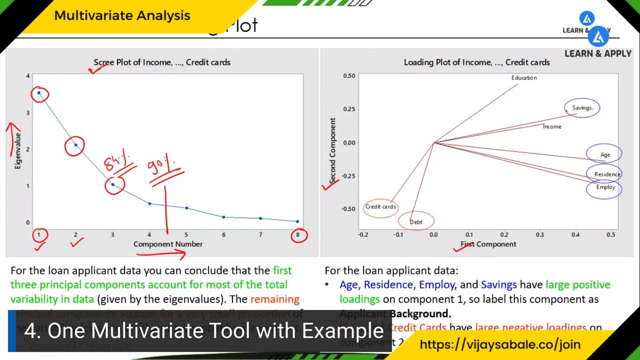 For example, we can see here savings: age, residence and employee. If you see, the length of all these four elements, or the variables, is same, so they can be grouped into the one category or one principal component: The debt and credit card. they are on the other side and we can also say: have the same length. 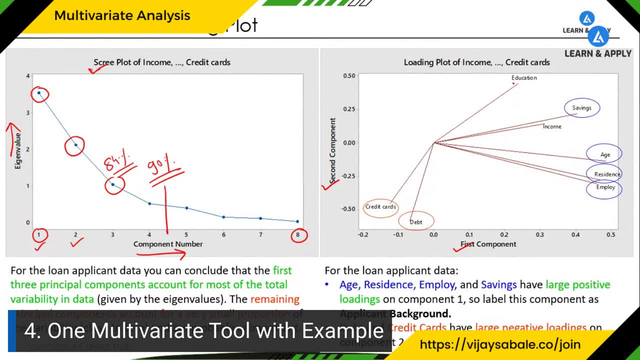 so they can group into the second principal component And the education and income we can see they are also having the similar length so they can group into the third principal component. So just by looking at the loading plot we can see how many groups we can have and into 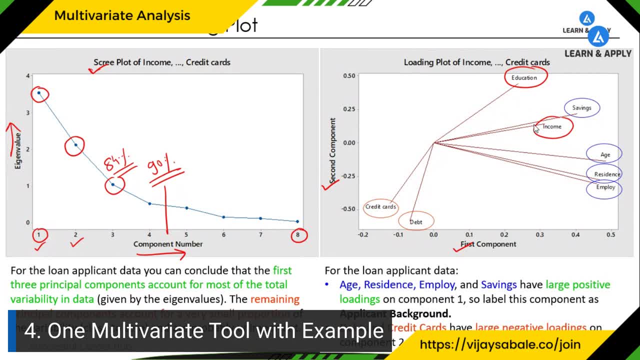 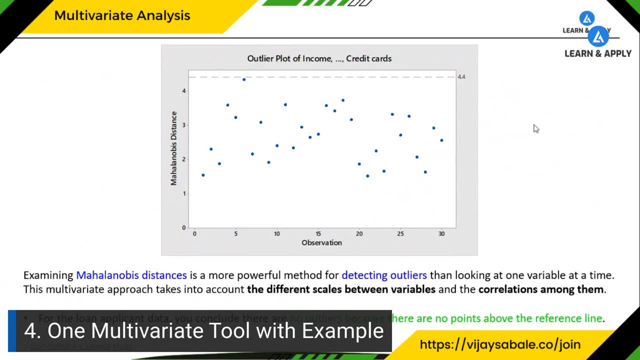 which or how many number of effective groups we can cover or we can divide our entire data. The next is about the outlier plot. This is very important because here we are going to use Mahalonobis distances method, In that if there is an outlier, 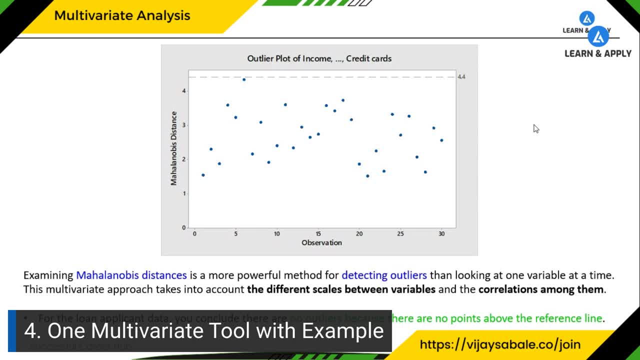 Now, what is outlier? Outlier means unusual observation. there is some problem or some error into the data collection. So if it is present, then there is one line that will be plotted by this outlier plot. This is based on the Mahalonobis distance. 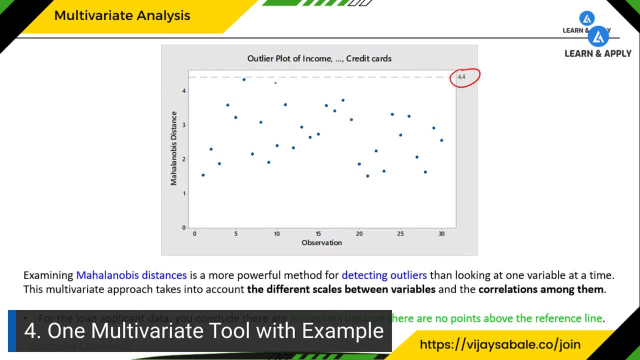 And if any points are passing this line, then we can call it as an outlier. The multivariate approach takes into account the different scales between variables And the correlation among them. for the lone applicant data that we are studying, we can conclude that there are no outliers because there are no points above the reference line. 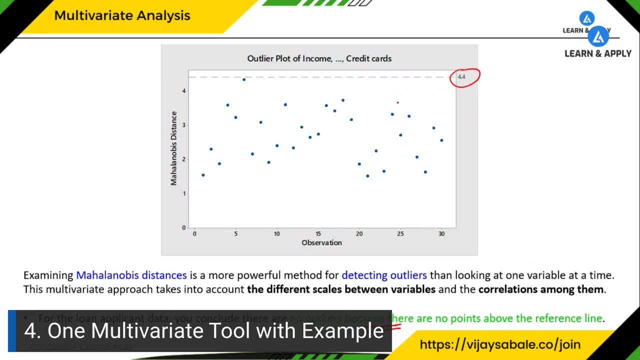 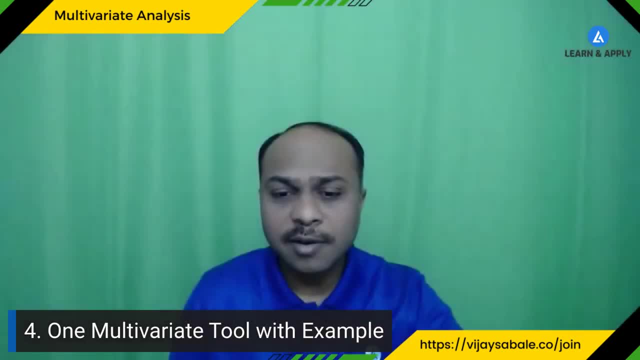 If any point that is going beyond this, then we can call it as an outlier right. So, based on this important graphs and outcome, we are having the very useful information that can be used to convert all the variables into meaningful principal components. A trick. 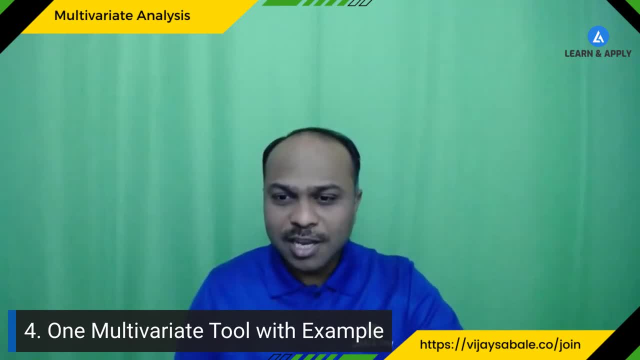 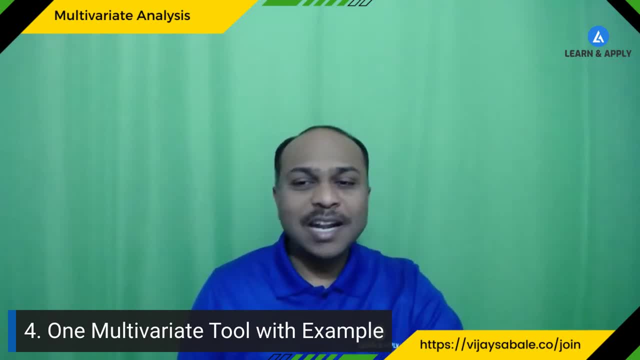 expert into SPSS. I'm using the Minitab and Sigma Excel to perform this analysis. I'm so sorry for that. I'm not aware about the SPSS. Thank you so much. Yes, we can use that into the SPSS. 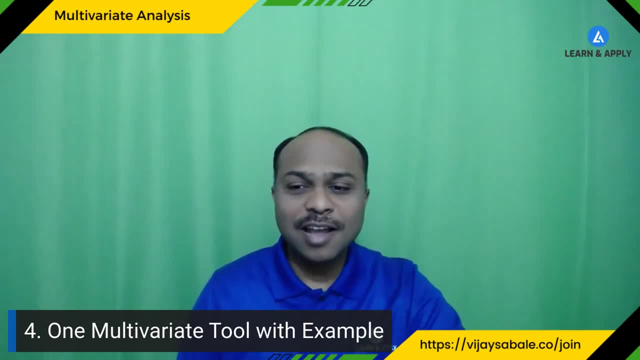 This multivariate analysis, But how to do that? I don't have experience on that. I'm so sorry for that. Thank you so much. Okay, So with the help of one practical example, we had also seen that how we can use this. 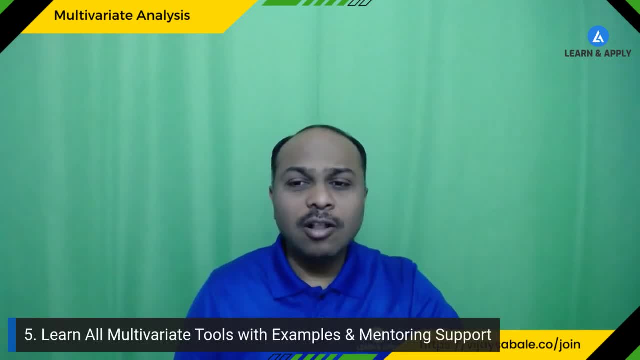 multivariate analysis. Now, if you want to learn all these other important tools, if you want to learn all the multivariate tools with the help of examples and mentoring support, just visit this link: vijayasabeco slash multivariate And we can learn, and you can learn all the important tools that I've explained, all the 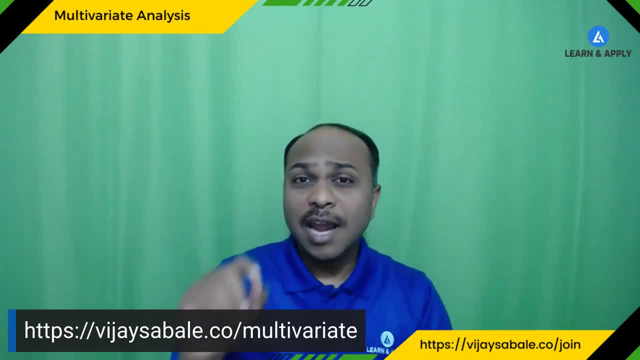 multivariate tools with help of practical examples, supporting data And, the most important thing, is my mentoring support. You will be getting the lifetime access to this content and still you are here. I can also provide you the one coupon code that you can use so that you can also get. 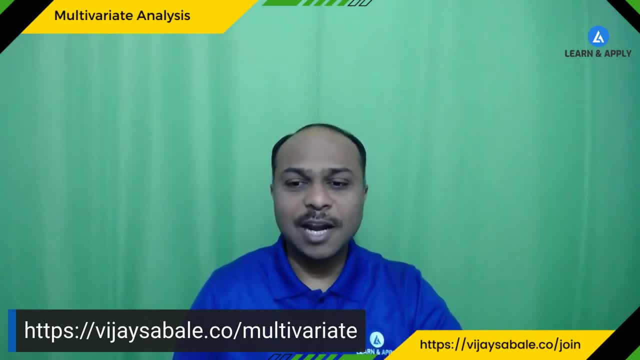 the 10% off on this, Thank you, Thank you. I can also provide you the entire program. Use the coupon code 10 start. Okay, I've also explained how we can learn all these multivariate tools with the help of practical. 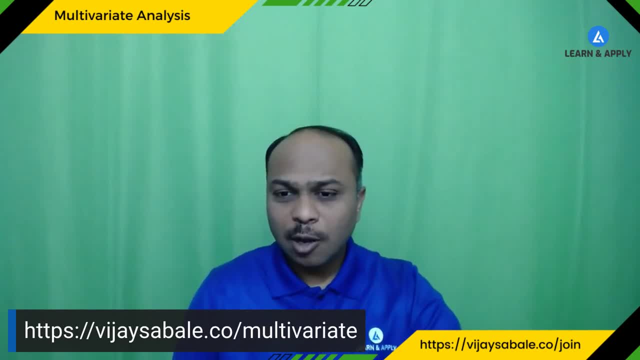 examples: supporting data and mentoring support. Now, if you're having any questions, please ask that question into the chat box. I'm ready to answer all your questions now. Please insert all your questions in the chat box. Please insert all your questions into the comment box or any comment suggestion that.